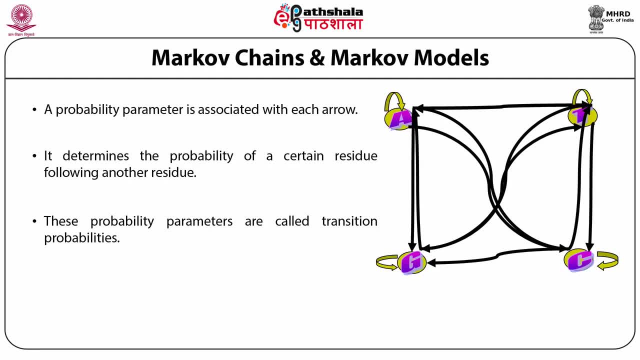 to the next state by a transition probability. So in any sequence of events, if I divide the set of events into discrete states And each state can have different outcomes with a set of probabilities, The probabilities of these outcomes of each state will be the emission probability and the probability that 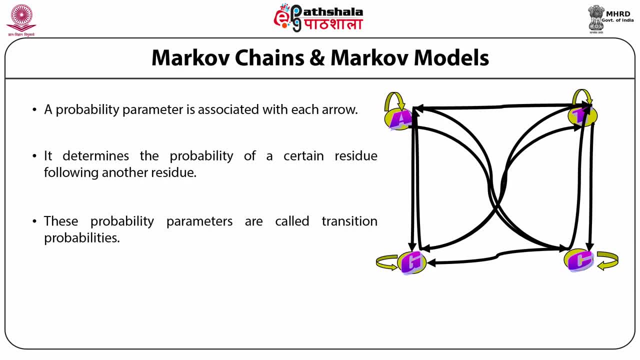 you will move from one state to the other state is the transition probability Now? it may be a simple sequence- In that case it is called a Markov chain. or it can be that from one state you can go to state this one or state this one. In that case you have. 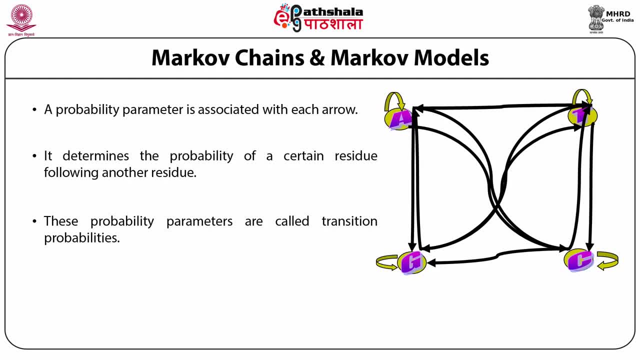 separate transition probabilities related. You do not have this, the chain, like this pattern, anymore. In such cases we will call it a Markov model. Again, let me reiterate: the Markov model is characterized by a set of states which are related by transition probabilities, and each state has a set of 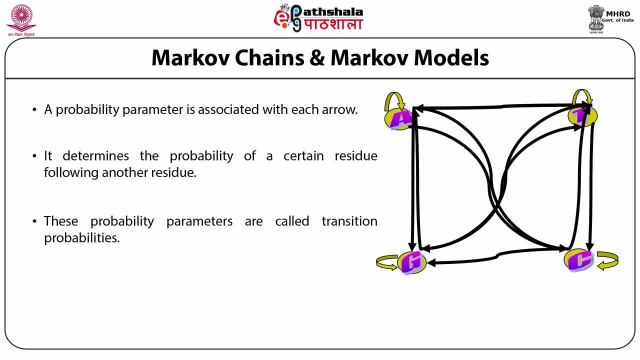 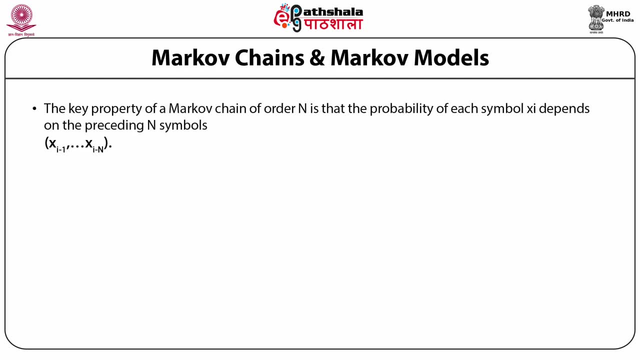 outcomes and the probability of each outcome are called the emission probabilities. So I have a set of states and I have a set of two kinds of probabilities: the transitions and the emission. Together I get my Markov model, Now the key property of a simple Markov chain of order. 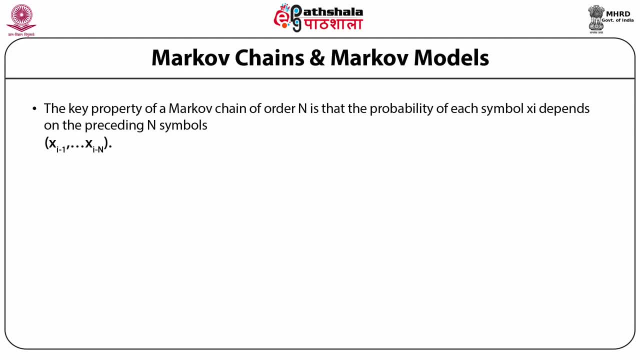 n, that is, I have n states in that particular chain- is that the probability of each symbol xi depends upon the preceding n symbols? which is there? Say, for example, if I can define that whether I get head in the fourth toss or not depends upon whatever I have gotten? 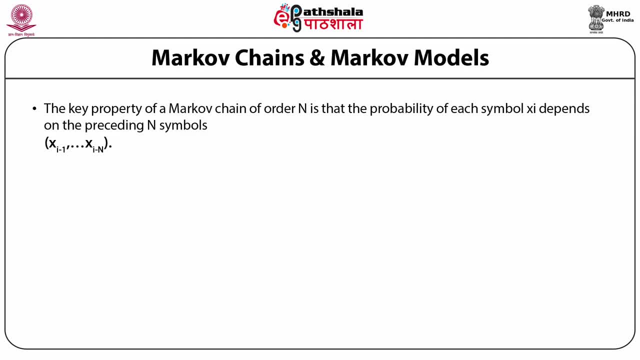 in the third toss, In the second toss, in the first toss, etc. Then such a kind of sequence of events can be modeled by a Markov chain. So now let us look at it a little bit more mathematically. Let us consider the probability that a particular sequence is obtained. So we will call it. 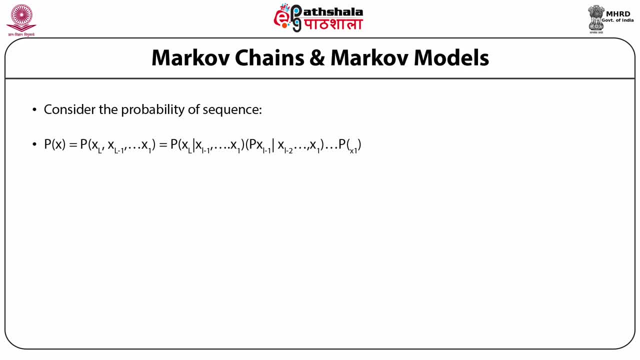 p of x and which, of course, depends upon p of x at L, L minus 1 until the first one, That is, the probability that I am in a particular state emitting something. This would depend upon the probability that I have visited all the previous states thus far in a certain 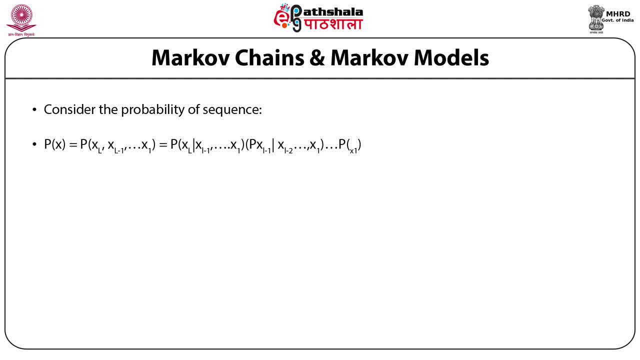 order. So this I can write as a conditional probability. This probability p now depends at the first state. I've got x given at L minus 1, L minus 2, and until the first state I have gotten some symbol right And times the product which is at L minus 1.. Whatever, 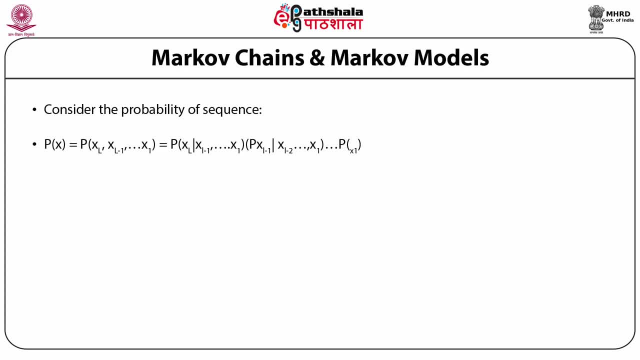 probability I've gotten is given to it. That means I'm required to preheat that particular given that, whatever I have got at l minus 2, l minus 3, and so on, so forth, Now writing this complex equation, let me remind you now of something called the Bayes. 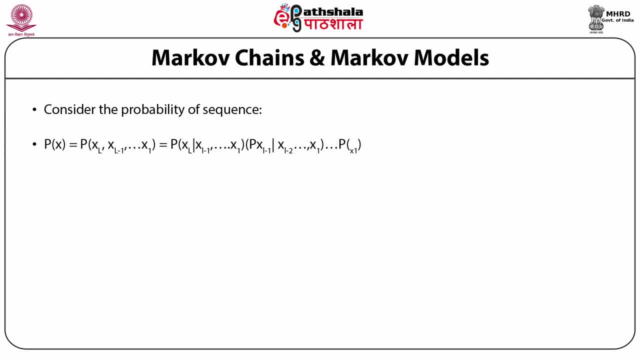 formula which is given as the probability of joint probability distribution of two events, p, x, y, is given by the conditional probability of p probability of x given y times the probability of y itself. Applying this, the Bayes formula, to the previous equation, right, I can now go. 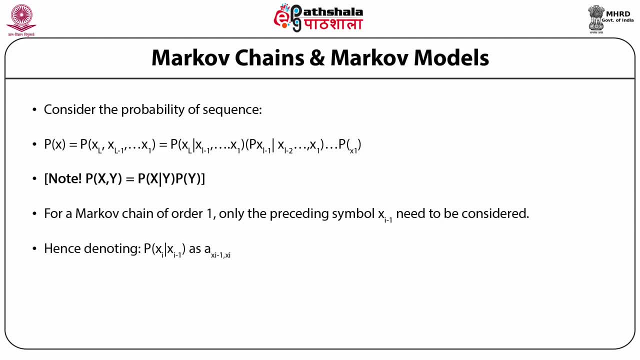 further. Let me make one more simplification, This long thing: probability of xi. given probability of xi minus 1, let me write it in a shorthand notation as axi minus 1 times axi. So, given that the previous equation now deduces to a simple product of probabilities which is given as p, x, 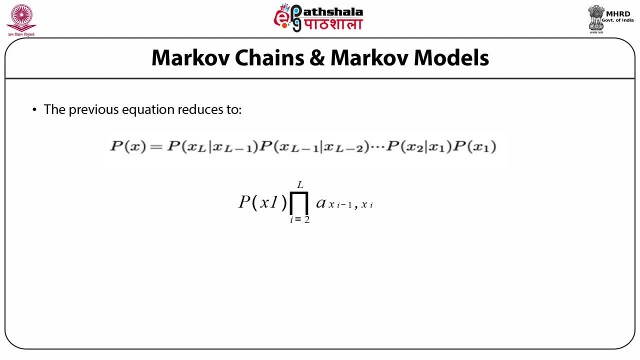 is now p x at position state. l is the product of whatever this probability is axi minus 1, axi minus 1.. For all i is equal to 2 to i is equal to l: all the states, So it's the product of all of these. 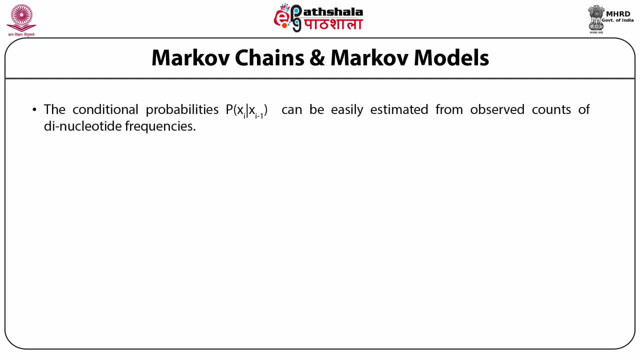 different probabilities. Now these conditional probabilities- p xi given, p xi minus 1- can be estimated from the observed counts which I measure from, by analysis of different Markov-like phenomena. For example, if I'm looking at a nucleic acid sequence, for example, I can always 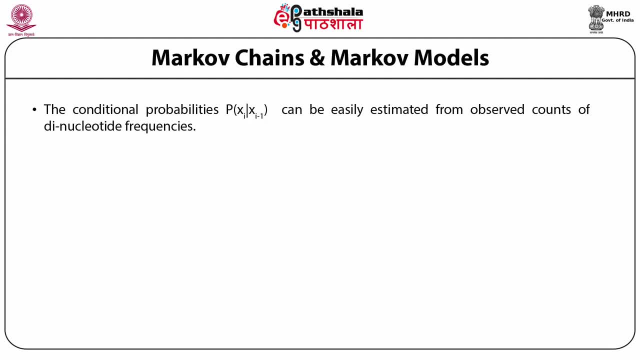 estimate p xi, given p xi minus 1 from the observed counts of the, say, dinucleotide frequencies. So I can extend the same formalism to higher order Markov chains. So we're going to make a third order Markov chain. So I have to count every trinucleotide frequency and so forth. So in this 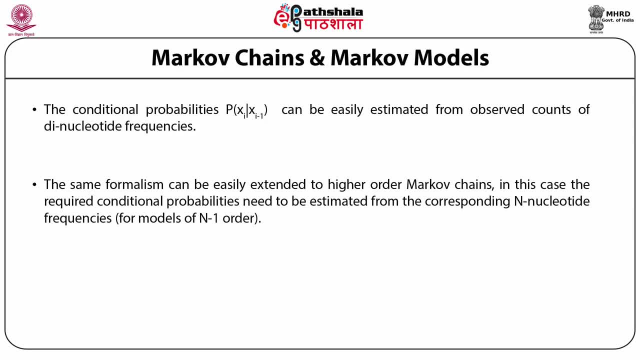 case, additional conditional probabilities needs to be estimated, And so with this I can create, for at least a DNA sequence, or even a protein sequence, I can create a Markov model, of any order for that matter. So here we call it the n minus 1 ordered. 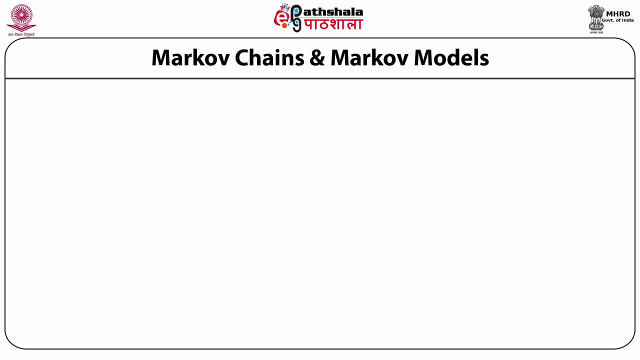 Markov models. Now, what use are these? The use of Markov models or Markov chains can be used to discriminate between two kinds of situation. Now let us say I have one sort of situation. I define it with a Markov chain. I have another sort of situation. I define it also with another Markov. 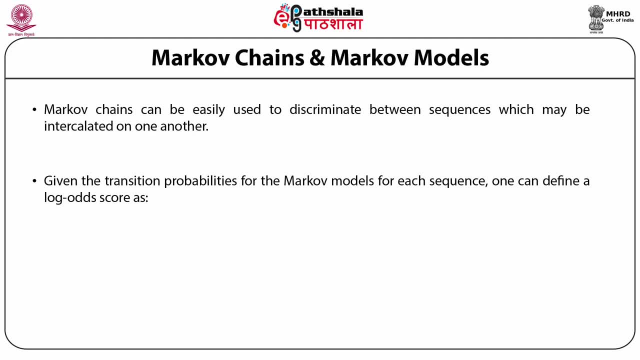 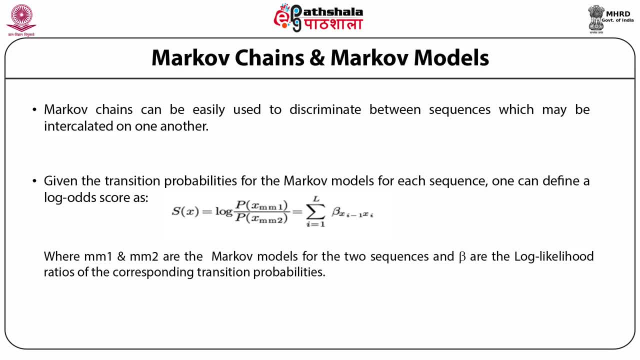 minus xj, where the beta xi minus xj itself is nothing but the probability of xi, given xi minus 1, and so on so forth. So this sort of logger's ratio can be fairly easily defined, which then tells me the probability that I either in this particular state or this particular sequence of 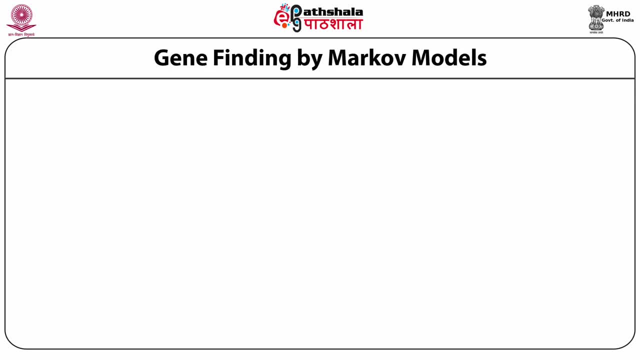 states or in that particular sequence of states. So where do we use this kind of concepts? One of the places where this is used is locating a gene. Now, why do I have to locate a gene? Nowadays, it's common practice to sequence the genome of an entire organism. Now, if I let's, if we take the 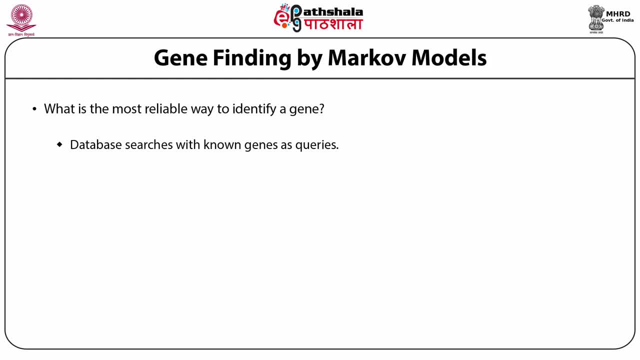 human genome, which is a huge sequence. right segments of it are actually protein coding genes. much of it are so-called junk dna or dna sequences with no obvious function. Now, given such a large genomic sequence, I need a method which is most likely going to identify to me those functional regions which 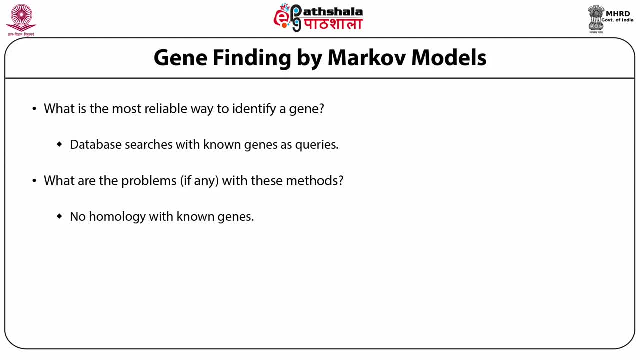 either code for protein or code for some regulatory elements, some RNA or whatever, right, and these are the likely genes. and how do I do it? Okay now, one way to do that is that if this particular gene, in this organism of interest, matches the sequence of some particular gene which? 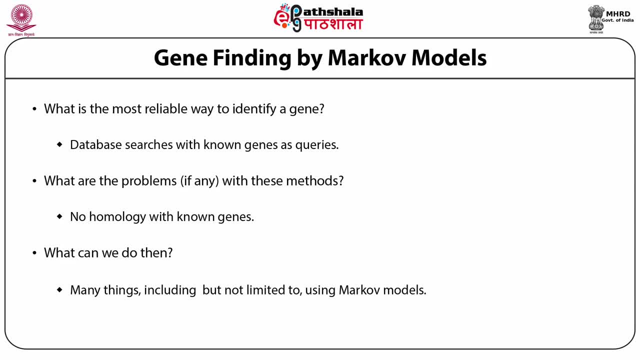 I know exists in another organism. I could use a homology based method, like, say, for example, blaster cycle last. But what happens if there is no such homology? I get an organism which is so strange, so rare, that its genes do not match with anything. What do I do? One of the things: 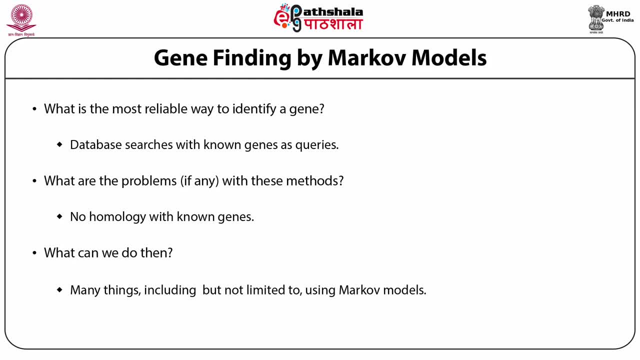 that I can still do is analyze with the help of Markov model. Let us see one of the uses of fixed-length Markov models. There's a program called GeneMark which finds genes from an unknown sequence using a fixed-length Markov model. Now why does one do that? Now, many times. 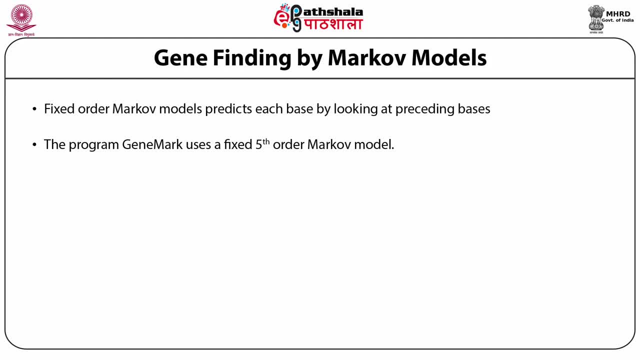 when you have sequenced a genome, you would like to see if there are any genes which are present there which you know about Now. of course, one way to do it would be do a blast search and see if it is similar to some other gene, But that may not always be possible, because there might be some. 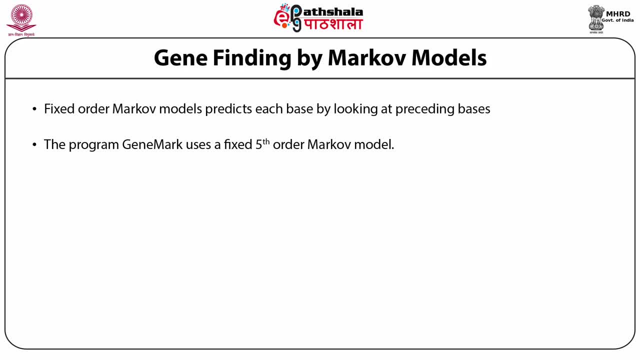 gene which is so different from others that there isn't any homologous sequence already existing in a database. In such cases, programs like GeneMark can be used. It uses a fifth-order Markov model. That means what it does is that it has the in a training set it has created the frequencies of all the. 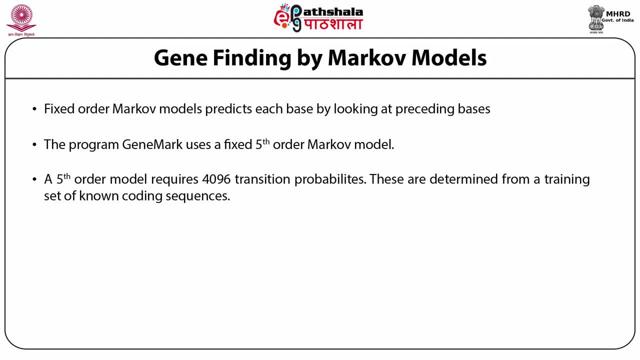 4096 pendant nucleotides. So, given a gene sequence, it looks at all the possible pendant nucleotides which are present in your unknown sequence and tries to see if their occurrence is predicted by the Markov model. So what happens is that the Markov model, which has been generated using this 4096 pendant, 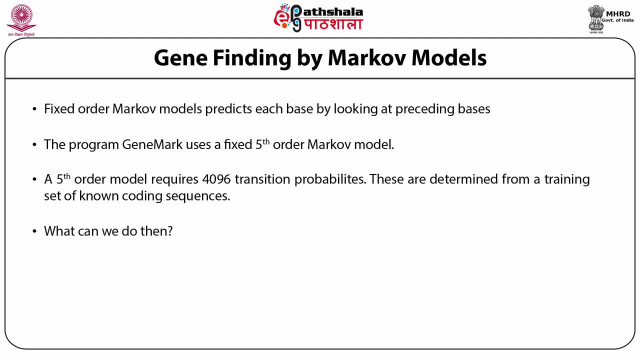 nucleotide transition frequencies. Now, while this might work, there are certain problems out there. Now think about it. There are only four single bases. There are 16 dinucleotides, There are 64 trinucleotides, 2056, 256 tetranucleotides and 4096 pentanucleotides. Now what would be the 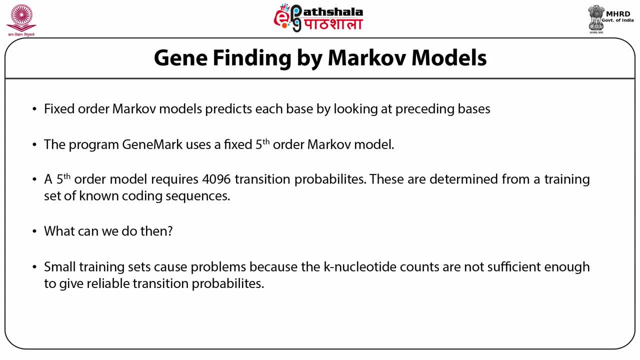 length of the DNA sequence database which is required to give me an adequate representation of these bases, or dinucleotides or trinucleotides, Obviously, since there are four bases, if I have a database of, let's say, 100 nucleotides or so, I would get a fairly good idea about. 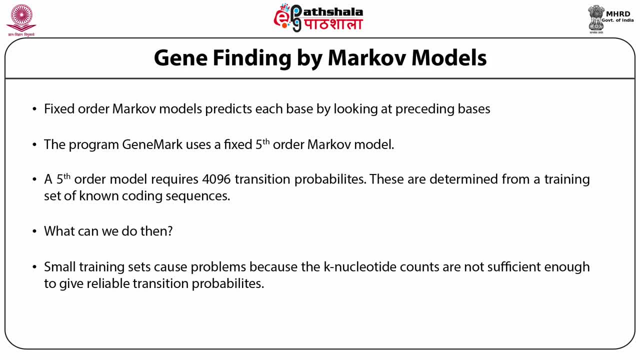 the relative frequencies of these four bases at least up to 1% accuracy. On the other hand, if I look at dinucleotides, there are 16 of them. So in a random sequence, if all of them are equally represented, just to get one dinucleotide. 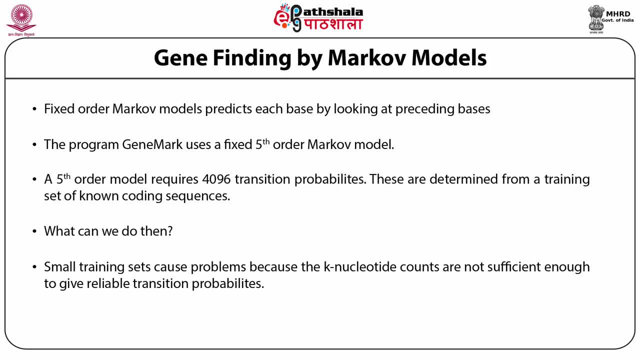 I must have at least 16 mer of DNA Now when I have so large 4096,. it may be that my database is not of sufficient length which gives me good enough counts of each of the 4096 pentanucleotides. 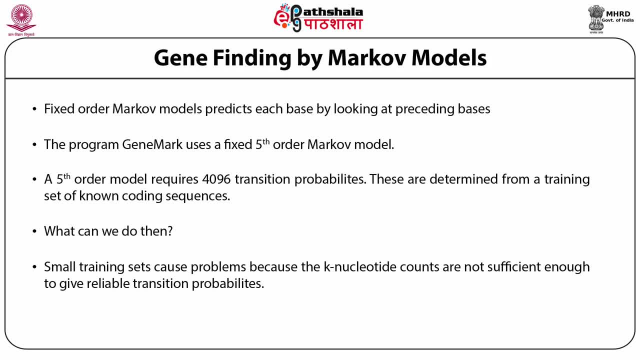 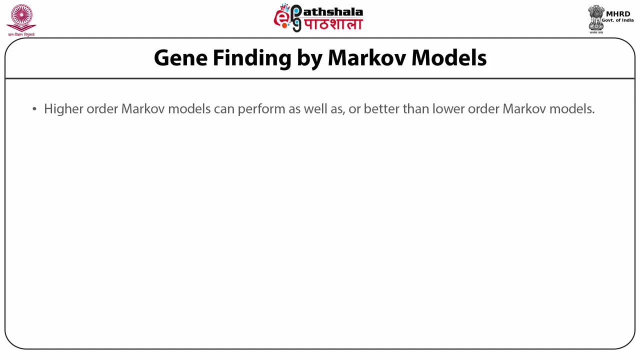 to be able to accurately construct the transition probabilities. So this means small training. sets cause problems because the k nucleotide frequencies or counts are not sufficient enough to give you a reliable estimation of the transition probability that's their frequency. So what does one do in such cases? Higher-order Markov. 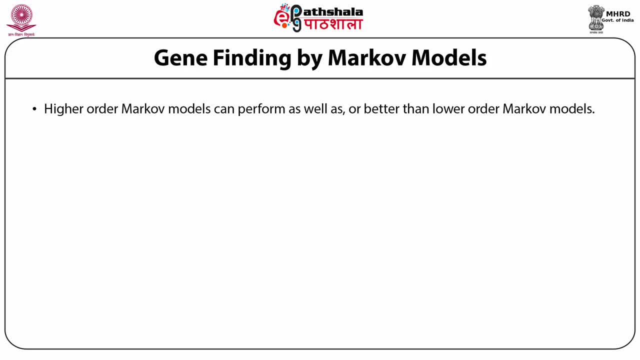 models, of course, can perform better than lower-order, that is, any model which works at 50-40� order frequencies generally performs better than fourth order, a third order, a second order. however, if your training set, from which you are training this markup model, you are obtaining the 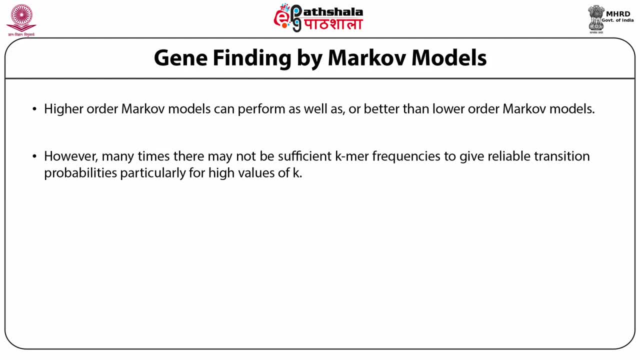 frequencies, the probabilities. if that's not large enough, then you cannot reliably create a high order markup model. so what you do in such cases? so wherever possible use as high as you can go. wherever not possible you come down lower in the order. so for example, if for 4096 pentane 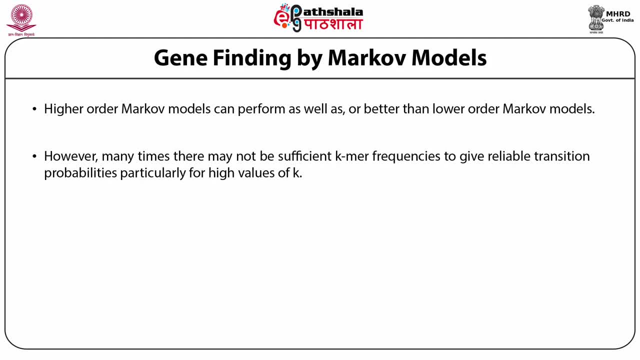 nucleotides, my database is, as a reasonable representation of, let's say, 4000 of them. so then i use it. but for the remaining 96 my database is not good enough. it's it's not big enough. so what i do? i move down to a fourth order markup model. now there are only 256 possibilities. 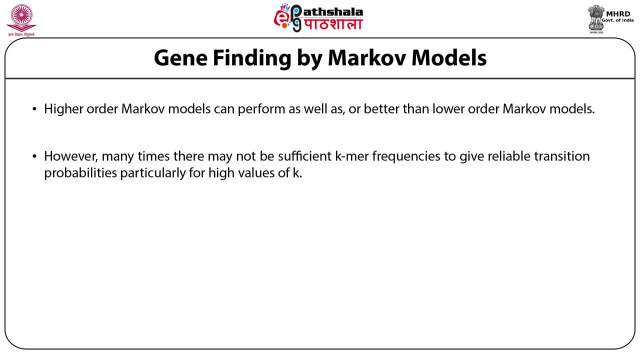 in fourth order. so a database which works well for a majority of pentane nucleotides definitely is likely to work better for tetra nucleotides and so on, so forth. so i come down one step below such kind of markup models which are not fixed in their order they go up to: 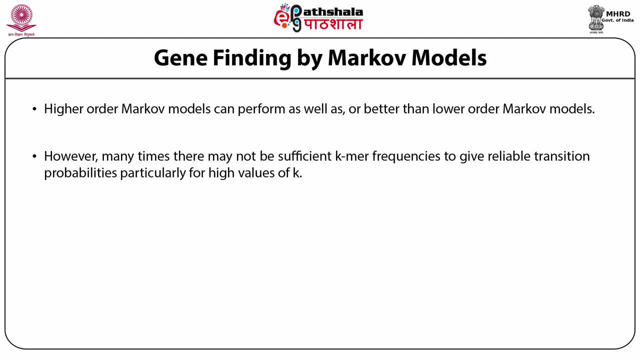 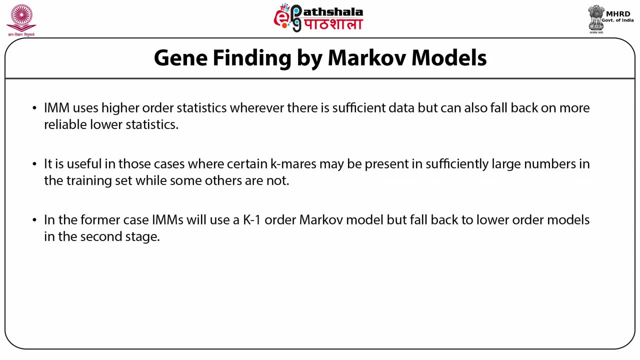 a certain level whenever possible, and then they come down a little bit whenever that thing does not happen. so this kind of markup models are known as interpolated markup models, and there are a lot of gene finding programs based on interpolated markup models. so in these ones we use higher 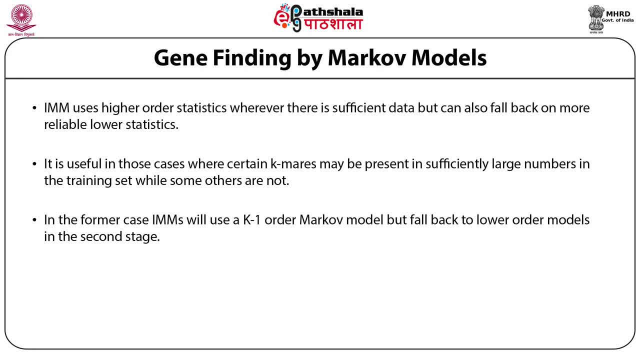 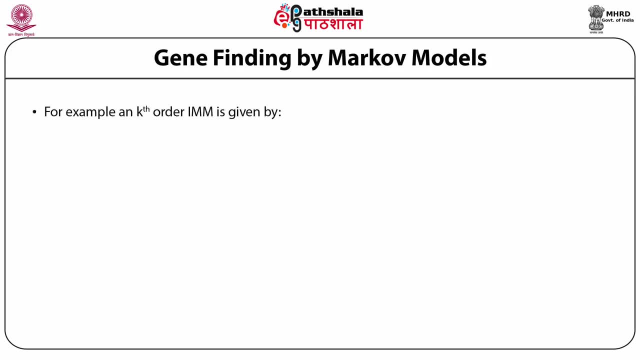 order statistics wherever there is sufficient data, but fall back to lower order statistics. so here is an example of a interpolated markup model of, say, kth order. so in this case my frequencies are lambda k wherever it's available. when not available, i use a certain by some, certain weight, i use a lower order. so i 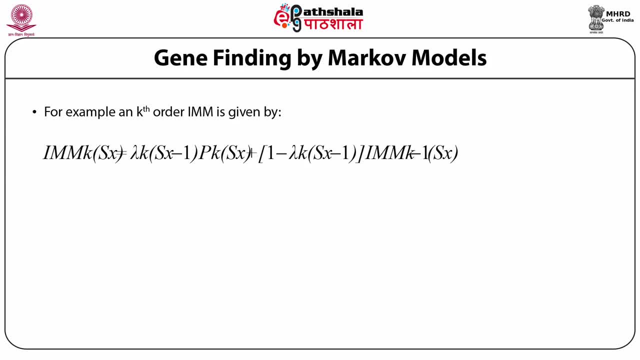 right. so in this way the lambda k is a weighting function. so where if possible, if i have enough statistics, i use the weighted function for the highest order possible. if i do not have, then i use a one order lower right for wherever it's not possible, and i can go on recursively. 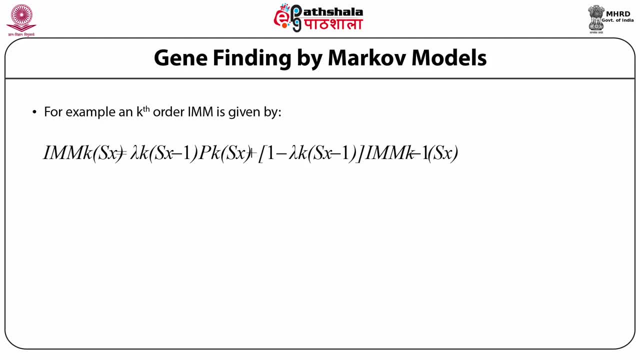 in this one, so that way i can go on as many orders below that i have to go. but the lambda k, s, x minus one is a numeric weight and this weight also needs to be trained. so the probability that a sequence is generated by a model is now given p s. the sequence given, generated by the model m, is given as the scores obtained from. 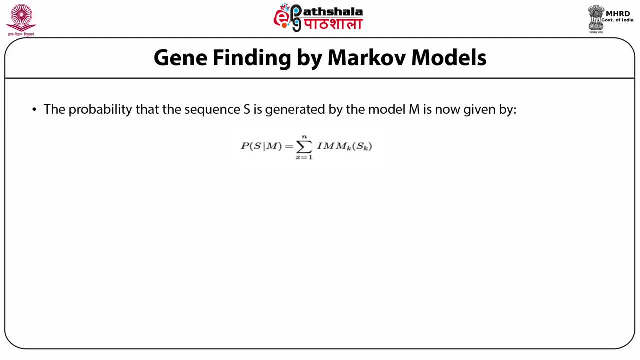 this interpolated markup model so, and it is a summation of the scores for every possible k length window. so therefore, the kth order markup model is just a linear combination of its lower order markup models. so one example of an interpolated markup model program is called glimmer and it's used for gene finding. so when applied to a 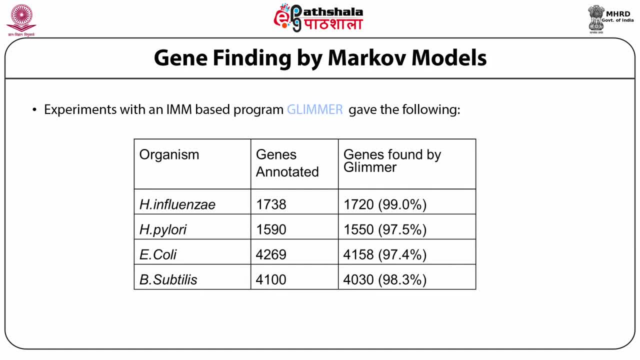 several bacteria, say hemophilus influenzae. it finds 1738 genes which are known to be there. 1720 of them are found out by glimmer, so gives you a 99% accuracy in most cases. as you can see that the accuracy is between 97 to 99%. 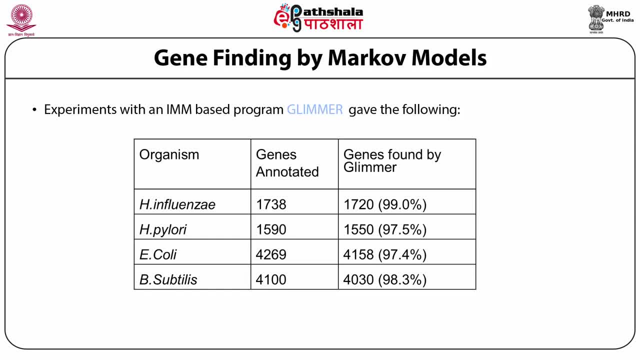 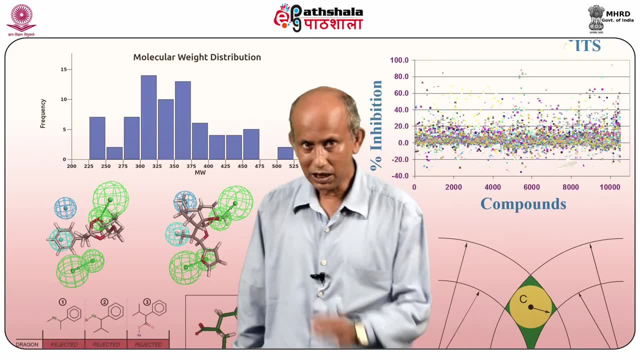 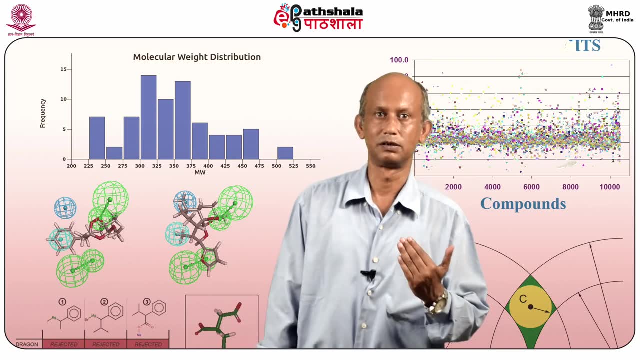 which is, I should say, a pretty good approach. so interpolated Markov models work slightly better than fixed-order Markov models now. but even these have a little problem, because here we're on the base of an assumption that I am looking for a gene which has a certain pentaneucleotide or tetra nucleotide. 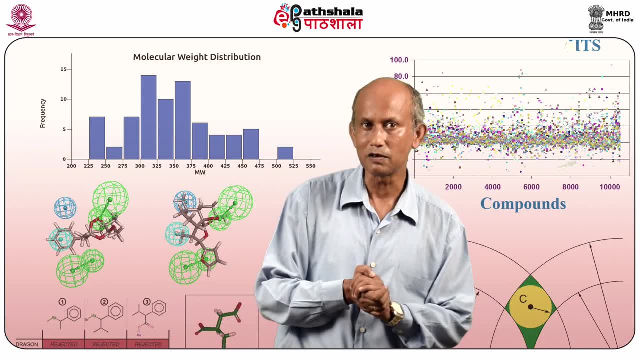 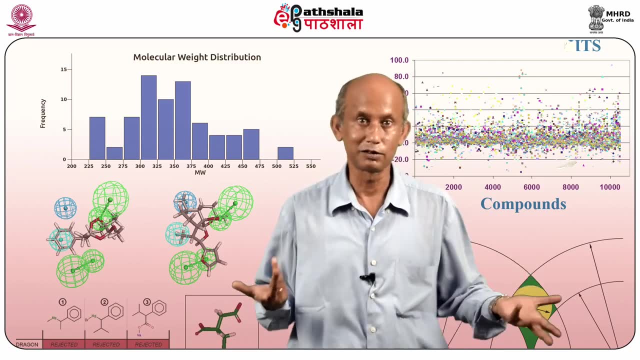 frequency and based on that I have created my Markov model. but sometimes I have created my Markov model, but sometimes I have created my Markov model. you know, even in your training set you don't know where the gene is there or where it's not there. then how do you even construct such Markov models? and an 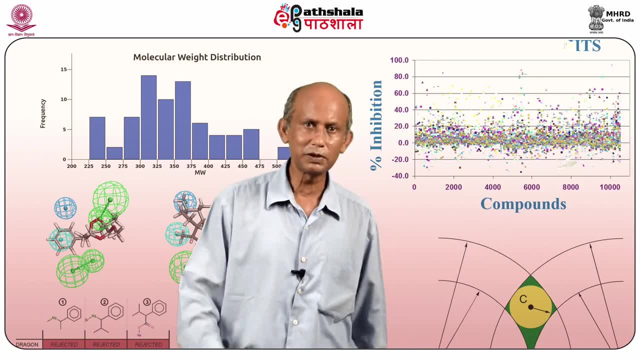 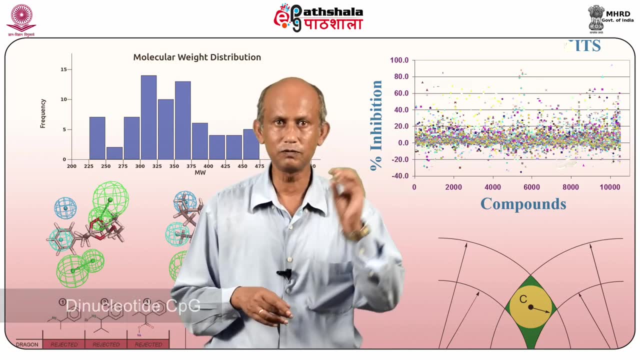 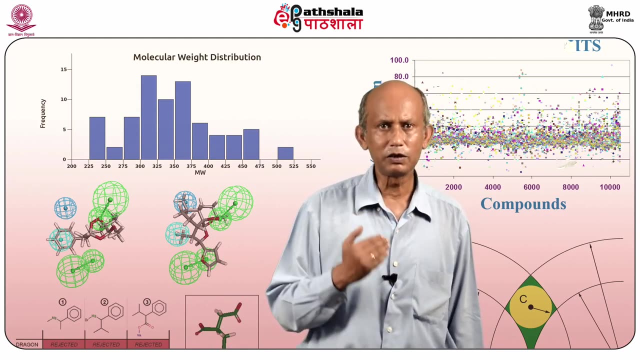 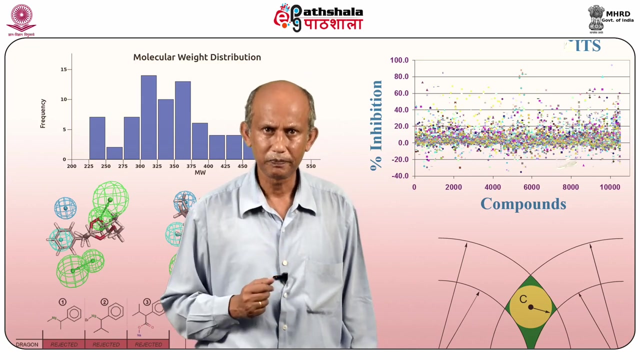 example comes here. say, for example, in the human genome there's this dinucleotide, CG, C, phosphate G, cytosine, phosphate, guanosine- we'll call it. CPG- is usually whenever it occurs, the cytosine nucleotide is typically modified by methylation, so we get 5 methyl cytosine, now 5 methyl. 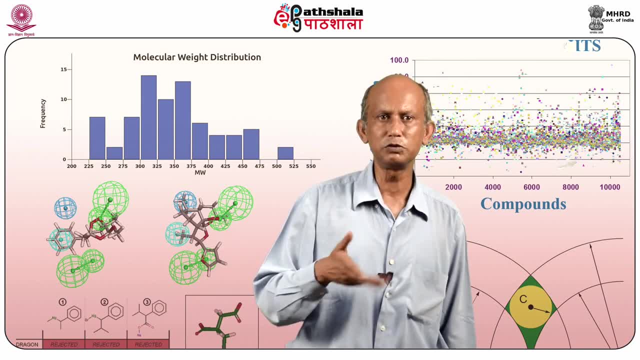 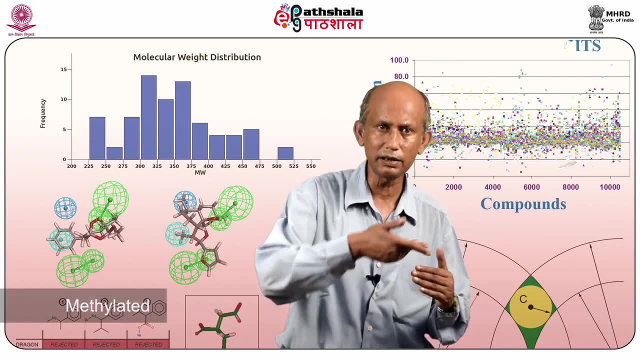 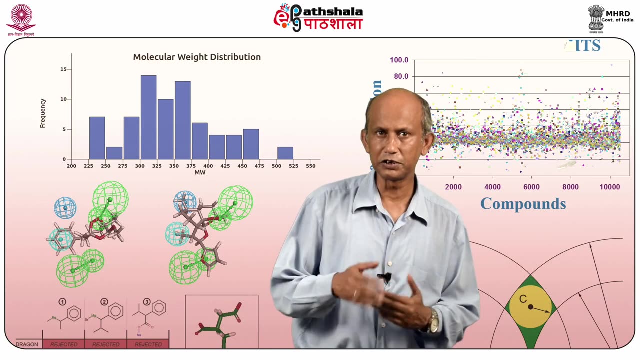 cytosine has a strong chance of getting mutated to thymine. hence you find the CPG sequence is rather rare, because it would have gotten methylated and then it would have mutated itself into thymine, as we have seen. the interpolated Markov models are fairly good for certain things, like, for example, gene finding. but 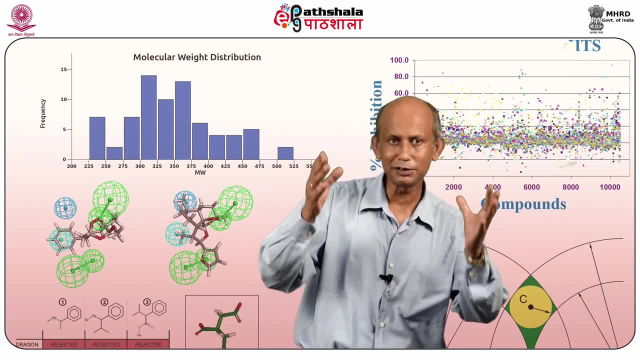 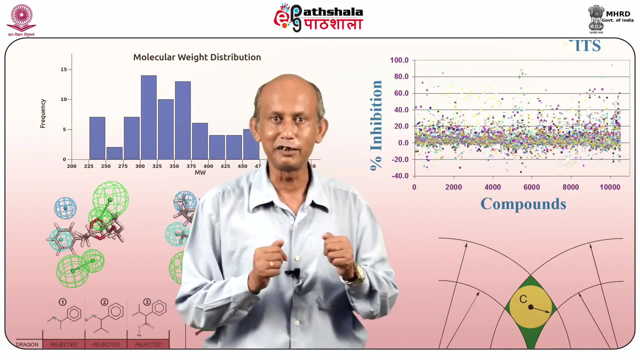 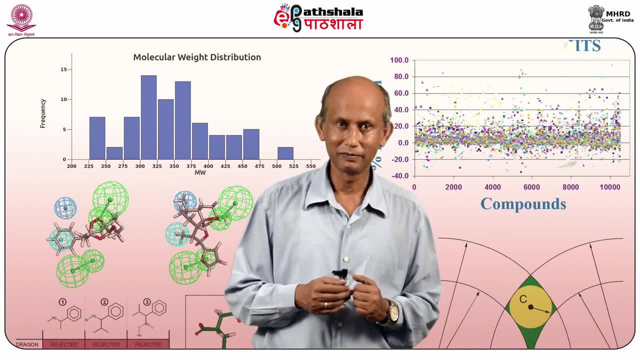 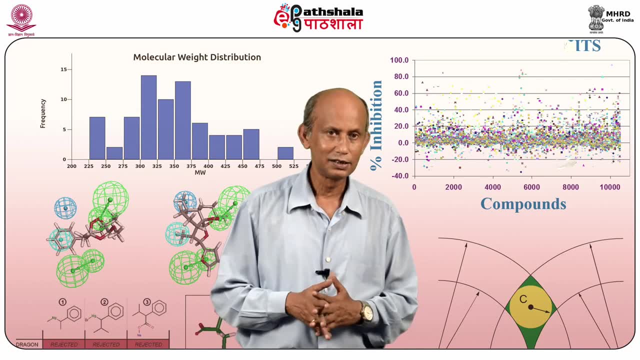 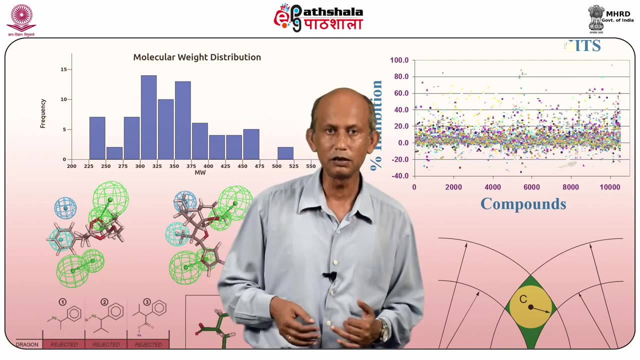 an interpolated Markov model to find such kind of genes. To give you an actual biological example, I'll take the case of the so-called CpG islands. Now, what are these? Now, in a human genome, whenever this dinucleotide CpG cytosine, followed by guanine, occurs, the C nucleotide is typically modified by methylation at the 5 position to 5-methyl cytosine- Now 5-methyl cytosines- they have a strong chance of getting mutated to thymine. Hence it is relatively rare to find the CpG dinucleotides occurring inside the genome. So generally you don't find them because 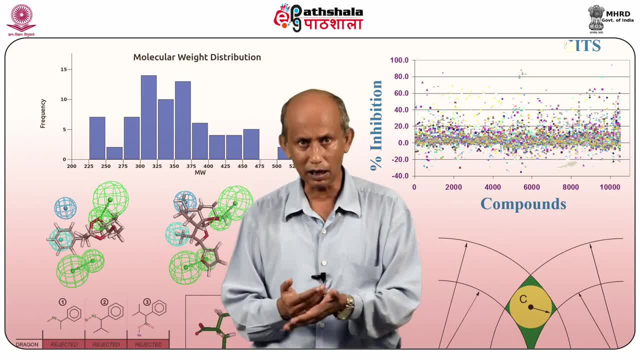 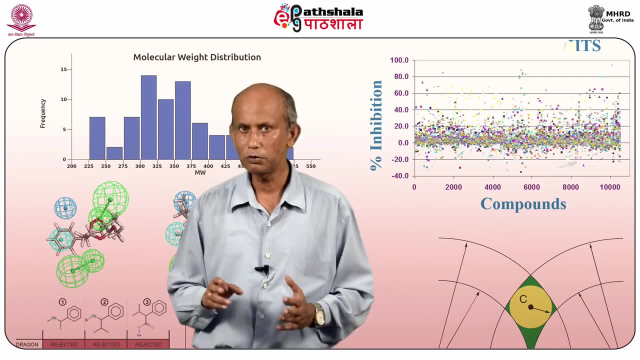 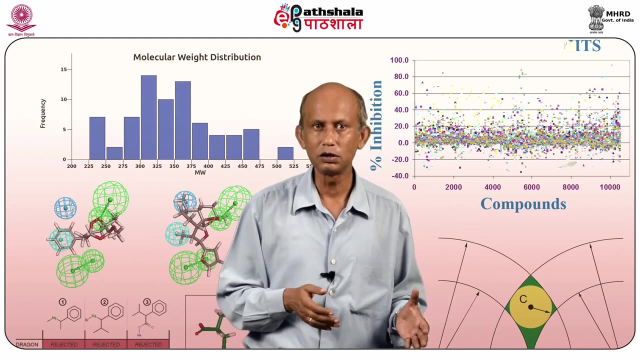 wherever they occur, chances are that the cytosine has gotten methylated and has mutated itself to thymine. For certain good enough biological reasons, which we know now, this methylation of cytosine is suppressed near certain important regions of the genome, namely in around promoters or transcription start sites. As a consequence, in such kind of regions which are promoters and so on and so forth, the frequency of CpG dinucleotides is rather higher, and these are called CpG islands. and typically CpG islands are only about few hundred to a few thousand bases long. Now, it is not to say that within the island you only 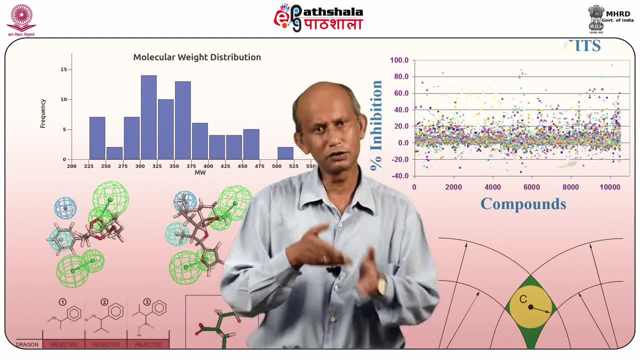 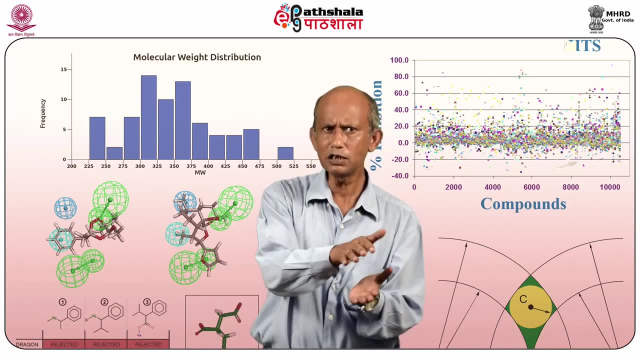 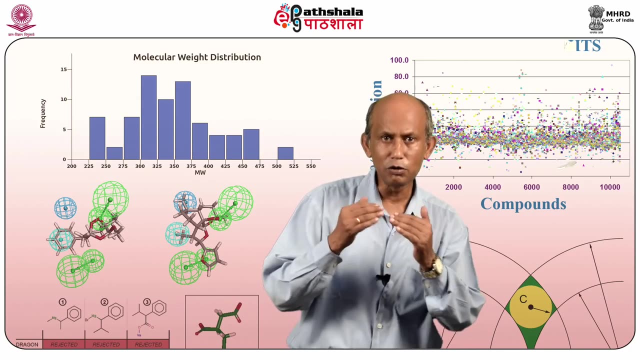 have CpG, you have also other nucleotides. and it is not to say that outside of an island you don't have CpG- you have. But it just so happens that within the island the frequency of the CpG dinucleotides are relatively larger. As a consequence, CpG dinucleotides are more common. 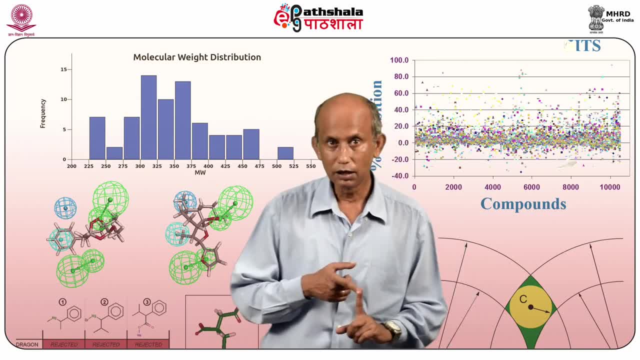 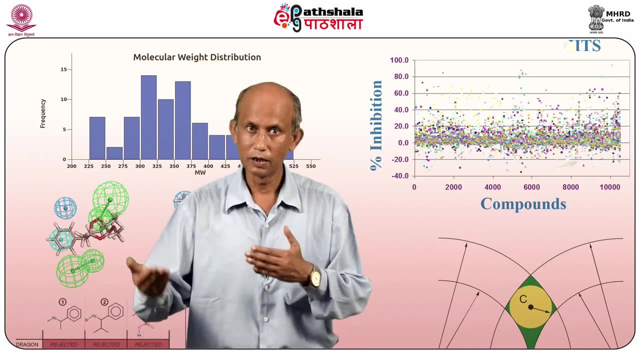 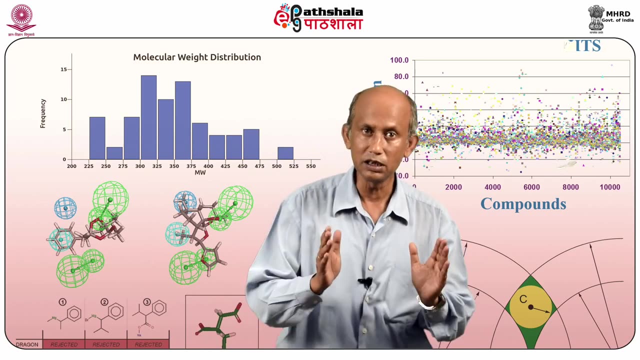 in these island regions. Now, this is not to say that within a CpG island, you will not find other nucleotides- Yes, you will. and it is also not to say that those parts which are not CpG islands you will not find CpG- Yes, you will. It just means that there are certain 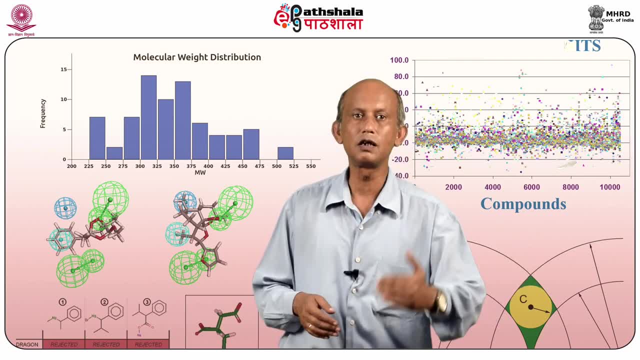 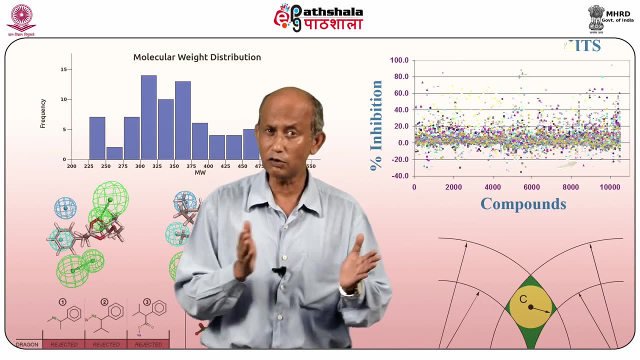 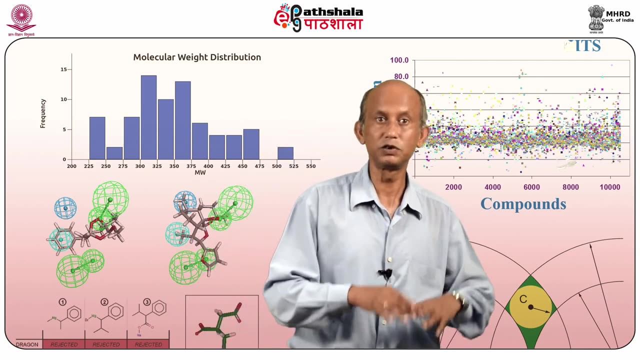 regions in the genome where the frequency of occurrence of CpG is a little bit more than certain other regions, and typically these islands are about few hundred to few thousand bases long. Now, because most of the time the CpG islands occur in these islands, which are important promoters or transcription start sites, 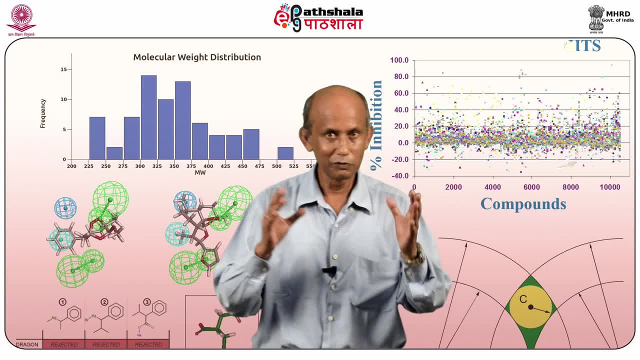 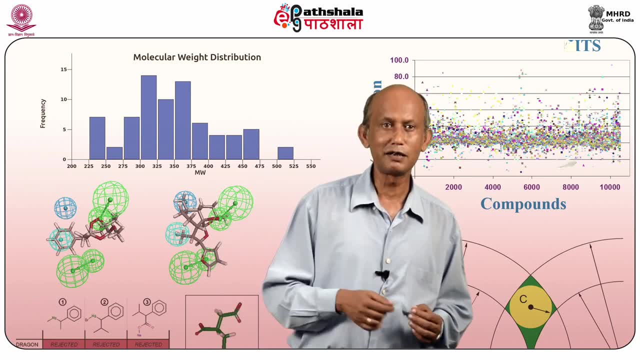 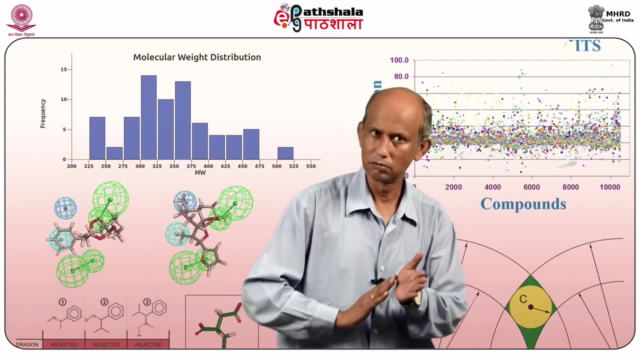 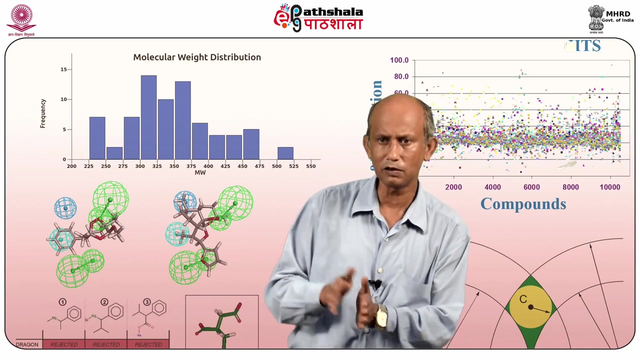 it becomes very important to locate these islands accurately. So we have the problem of identifying the CpG islands in a long, unannotated sequence. One way to do this would be to set up two different Markov models, one for CpG islands and one for non-CpG islands, The same way we do that for gene finding. We set up one Markov model. 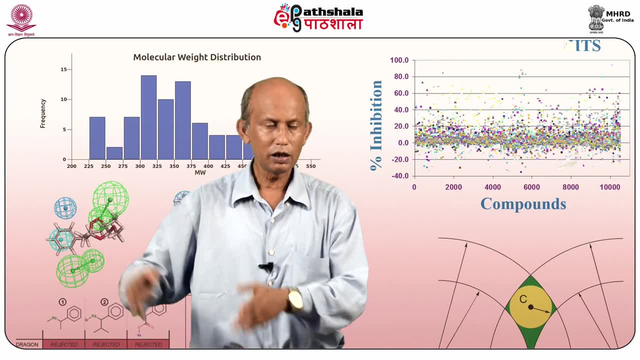 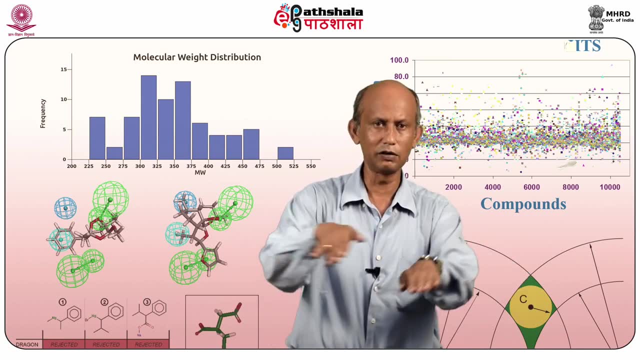 interpolate your Markov model for genic regions, which we know and we set up, and try to create another Markov model for non-genic regions and then, given an unknown sequence, we run it through both. We calculate a log- odpowied ratio and see if it is above a certain threshold. We can do that. 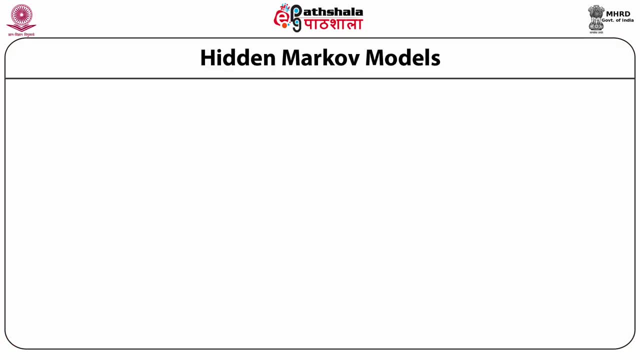 here as well, However, there is a little bit of a problem. So again, let me reiterate: given a text sequence, a test sequence, we run it through two separate Markov models: one for CpG islands, one per non-cpg island. take the logout score and get this logout score s and one can then use this. 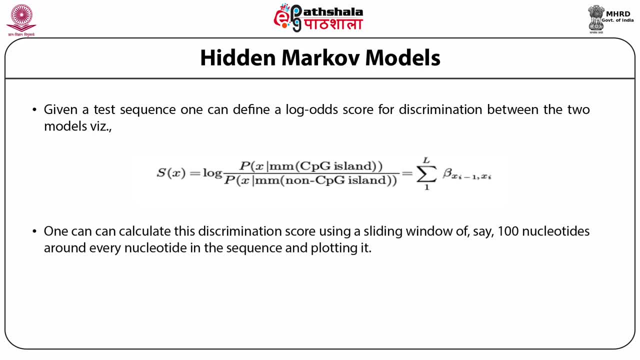 discrimination score in a sliding window of, say, 100 nucleotides and then plot it and whenever this discrimination score is higher than certain threshold, we claim that this is a cpg island. but this approach has a little problem at the boundaries between cpg islands and the non-cpg. 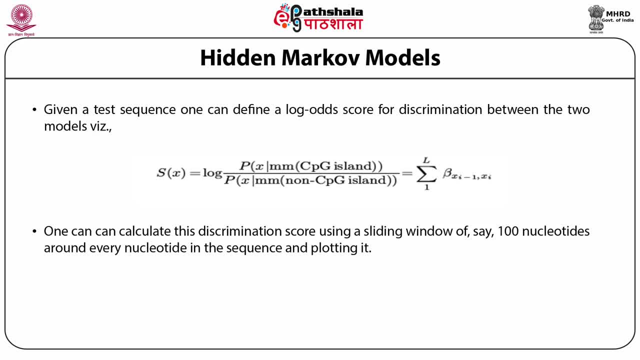 island is not clearly identified, because if your window length is rather big and as you are sliding your window, as you move from the boundary of cpg to non-cpg, your score is slowly, in a smooth fashion, it is coming down. so this does not allow you to identify the boundaries, and most of the 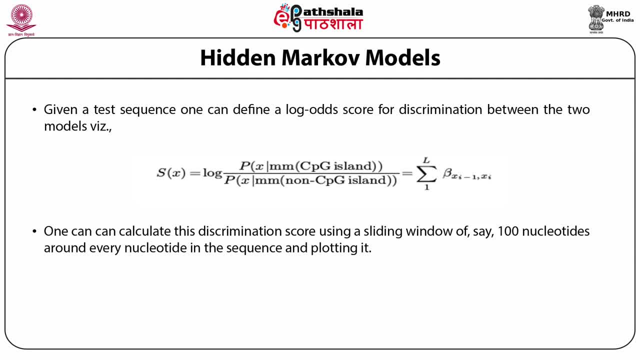 time. that is very important. so the length of the window reduces the sharpness of the signal. so what do we do? one approach is now to build a single markov model for the entire sequence, which contains both this markov chain, one for cpg, one for non-cpg. so given two markov models, 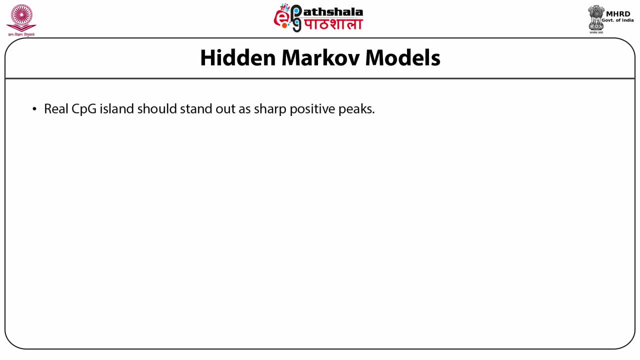 mark of chains, rather one for cpg islands and one for non-cpg islands. i can define this discrimination score, which is a logout score, so i find out the probability that a particular sequence belongs to a cpg island or it belongs to a non-cpg island. take the ratio, take the log. 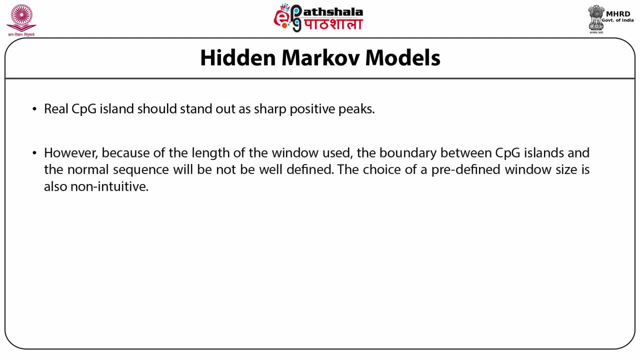 and i get this score. now i can calculate this score in a window and then i can slide this window looking for the value of the score. in a cpg island it should be rather high, in a non-cpg island it should be rather low, and as i pass from a cpg island one to the other it should come down as. 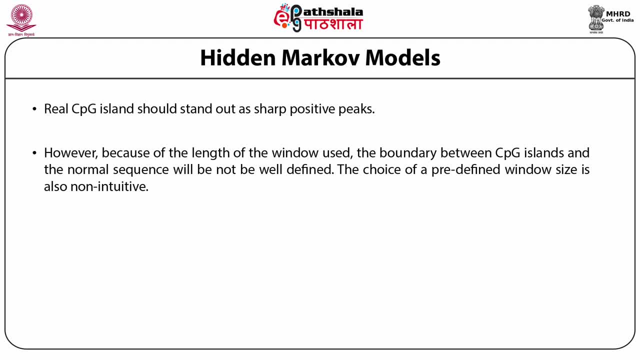 it should remain half and then it should come down. unfortunately, because this window length is rather large, what would happen at the boundaries? it is not going to come down very sharply, it's going to come down rather slowly, which would mean that i have a difficulty in identifying the 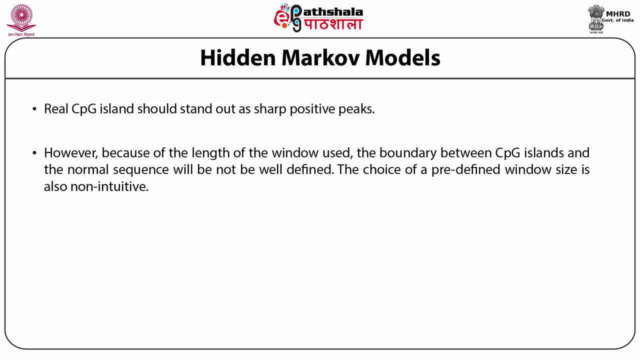 boundary where one cpg island ends and the non-cpg island region starts. now what can i do for this? one approach would be to build a single markov model, not two separate markov chains, mark models for cpg and non-cpg, just a single markov model for the entire sequence which incorporates information. 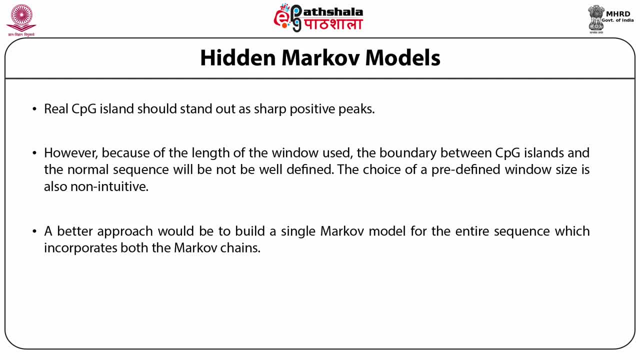 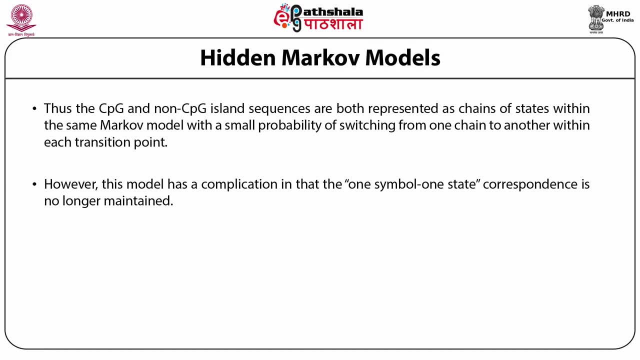 both from the cpg islands as well as the non-cpg islands. from the non-cpg islands. however, using this sort of a combined approach, there is one complication that earlier i had this one symbol, one state, that is either a, t, c or g, which are the symbols? they 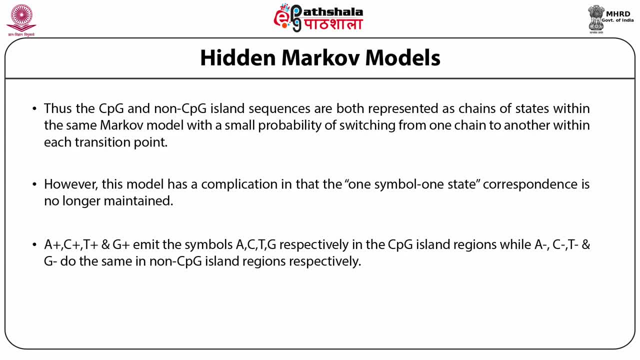 either belong to cpg or they belong to non-cpg. there was no way they could have mixed up, but now that i am having both the chains in, incorporated in one, i have a situation. i might have an a, c, g or t which may be part of a cpg island, or the same things may be part of a non-cpg island. so one way. 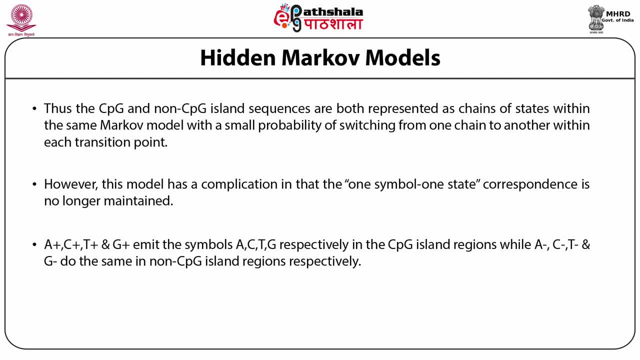 to avoid this problem that i define two kinds of bases. i define a plus c plus, t plus and g plus, which are the same thing- adenine, cytosine, thymine and guanine when they come from a cpg island or i- and i also defined a minus, c minus, t minus and g minus for the same four bases, but this time coming. 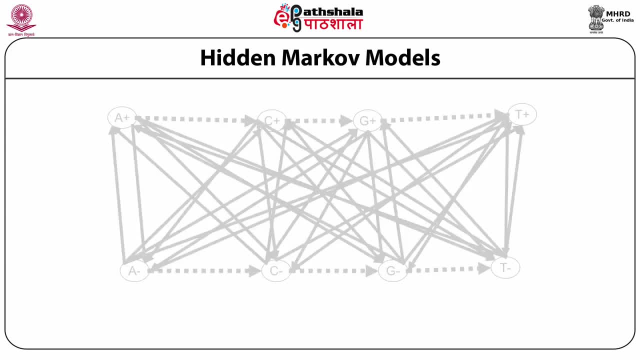 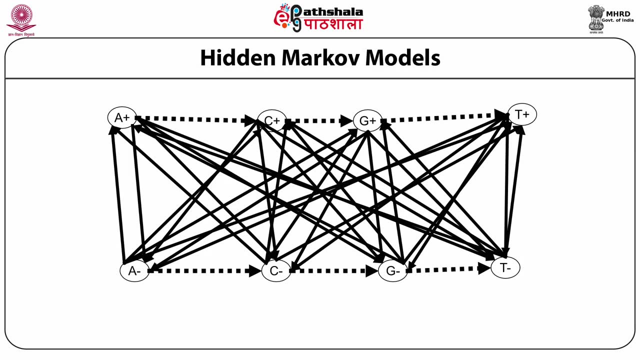 from a non-cpg island. so this is the overall shape of my markov models. at the bottom i have the non-cpg islands: a minus c minus, g minus, t minus. at the top i have a plus, c plus, g plus and t plus i have transition. 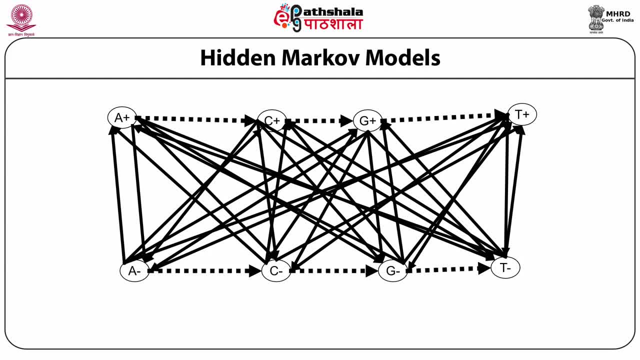 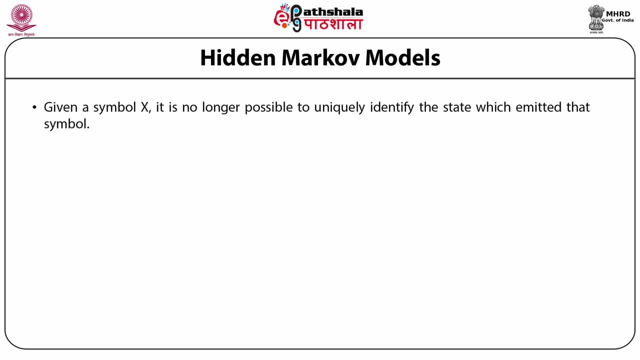 probabilities for every state going to every other state. now, given a particular base x, it is no longer possible in this kind of model to just identify whether it is coming from a c p g island or it is coming from a non-cpg island. so in this kind of situations the underlying states 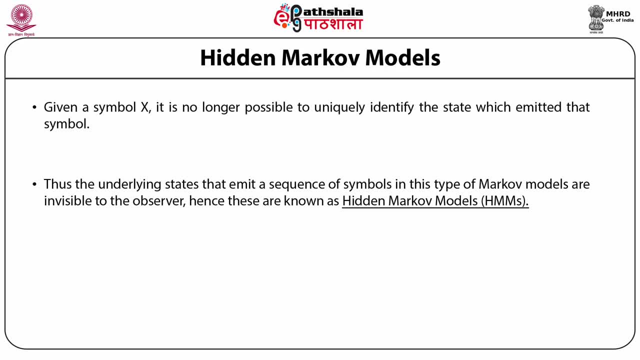 which is emitting the sequence of symbols is actually invisible or hidden from the observer, and hence this sort of markov model. we will call them hidden markov models or h m m s. now, whenever we are dealing with h m m's, we can ask certain questions. 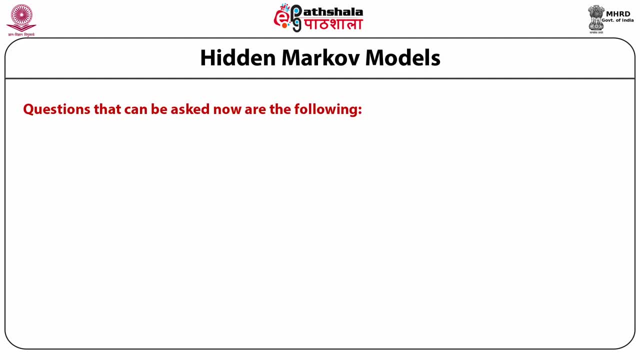 now, what are these questions? so one of them is like this. the double question is: q is to what do we take an observed sequence O which is made up of a sequence of symbols O1,, O2, O3, till O, n, and I have an HMM lambda. Now it has its own parameters. the emission probability is A. 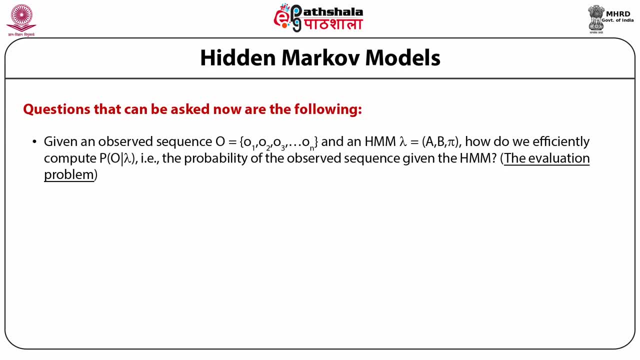 transition probability is B, there is a starting probability, pi, and so on, so forth. So I have an O, which is the observed sequence made up of symbols O1, O2, O3 till O n. I have an HMM- I define it lambda- which has its parameters A, B and pi. So the problem here is: how can I? 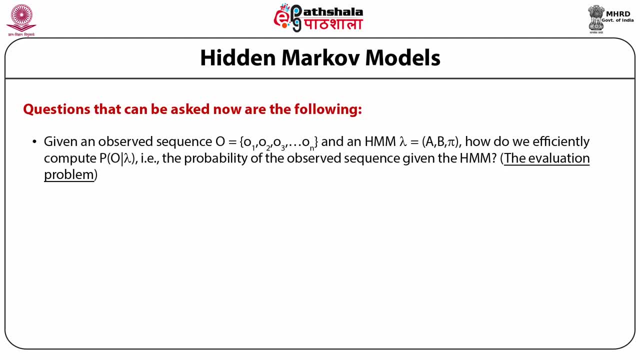 efficiently compute the probability of observing the sequence O, given the hidden Markov model lambda. So, given a sequence and a hidden Markov model lambda, I simply ask the question: what is the probability that this sequence could have been emitted by this hidden Markov model? Now, 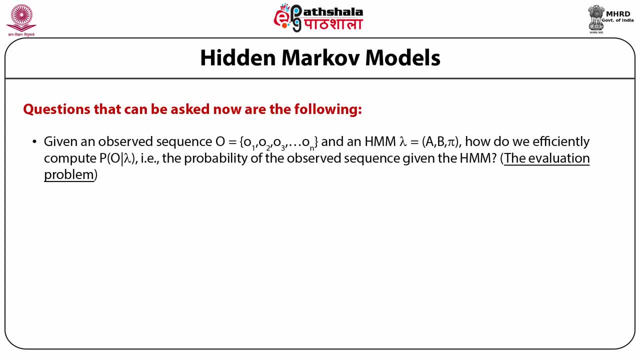 this kind of a question or a problem. we'll call it a evaluation problem. The second question which you can ask is that, again, let us take an observed sequence: O made up of symbols O1,, O2, O3, till O, n, and again I have. 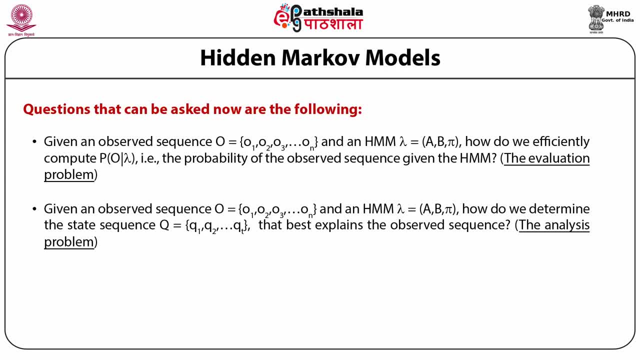 a Markov model lambda with parameters A, B and pi. Now I can ask this question. now that, can I determine a state sequence? that is a sub part of my hidden Markov model, right say, which I'll define as Q, with the state sequence O. Now I can ask this question. now that, can I determine a state sequence? 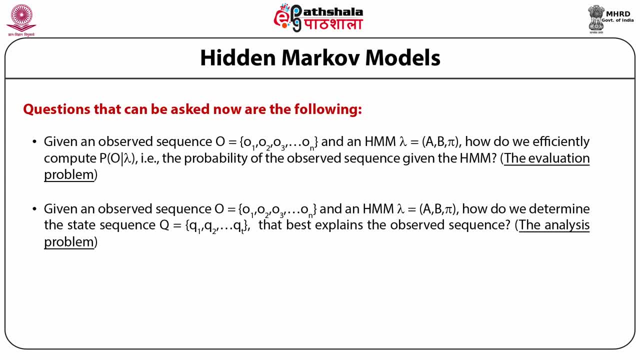 Q1,, Q2, Q3, which that sub part best explains the occurrence of the observed sequence. So I might have a very complicated hidden Markov model. but I'm asking: is there a subset of that hidden Markov model, is there a Markov chain within it which is best capable to explain with the largest? 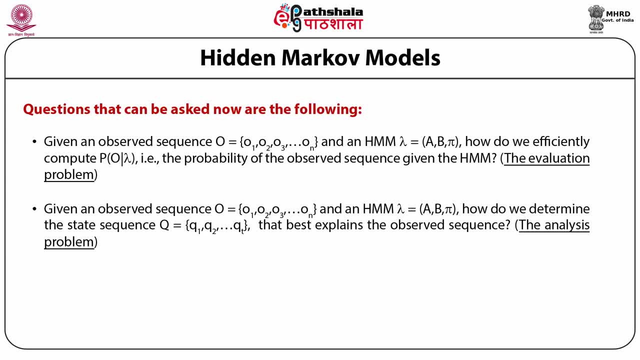 probability, P, O lambda, given my observed sequence, O right, This is called the analysis problem. And then, finally, the first two problems will even occur only after I have had created a Markov model right. So the last question I'm now bringing it should have been perhaps the first question- is. 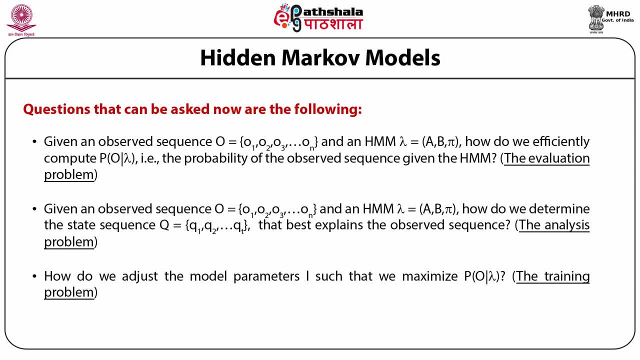 how do I train a Markov model? that if I have a lot of sequences and I want to create a Markov model lambda, how do I do it? and that, of course, is the training problem. So in the next few slides I will try and tackle each of these questions in order. 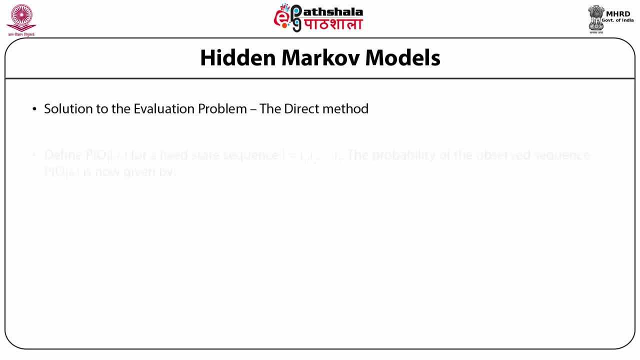 Let's try to solve the evaluation problem. Now let me define the probability of having the observed sequence given by a hidden Markov model, lambda, which has the following state sequence: I again comprising of I1, I2 and IT. Now this probability, P O given lambda, is given by the summation of the: 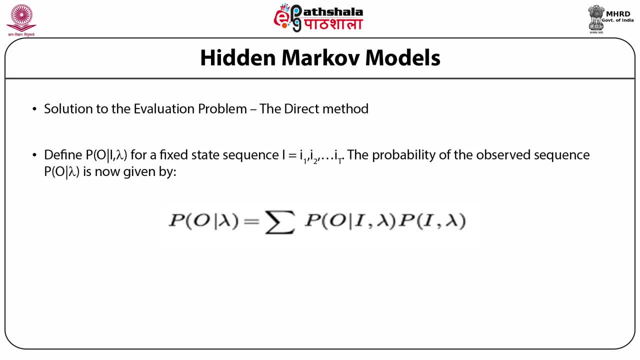 probabilities of P, given O, given I, and lambda times the probability of I and lambda. We further defined an initial state, let me call it pi i and for which the probability is pi okay, so a starting state which is not part of my sequence, and I defined a transition probabilities aij, which 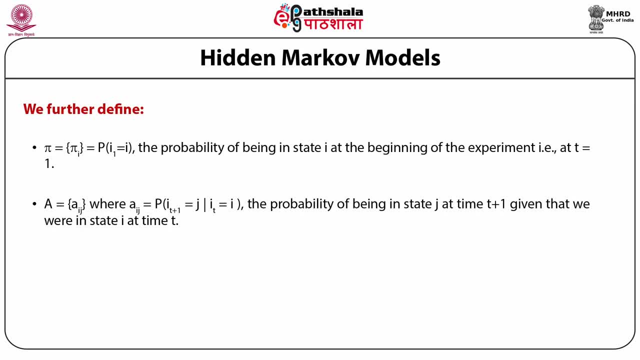 is given the probability that I will move given state i. the t-th state is i. I move from t plus one state will become j. So and again I define a parameter b which says: is that, what is the probability of observing the symbol vk if we are in a state j? that is the emission probability. So again I have a starting probability, pi. 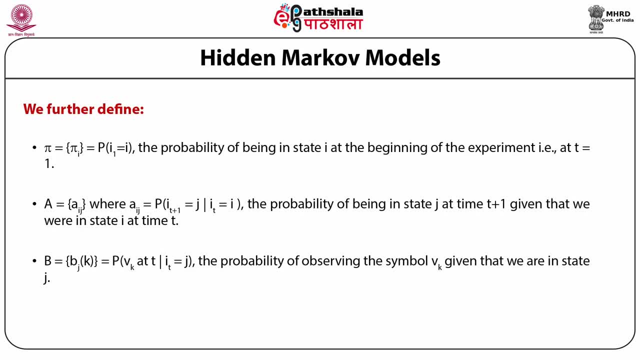 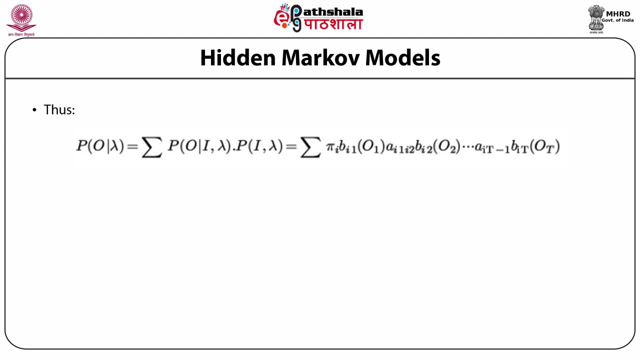 then I have a transition probability, aij, and I have an emission probability, b or bj. Now, given all that, now it turns out that the probability I'm looking for is given by the long equation summation of pi times b, times O1, aij to t, blah, blah, blah, blah, blah. 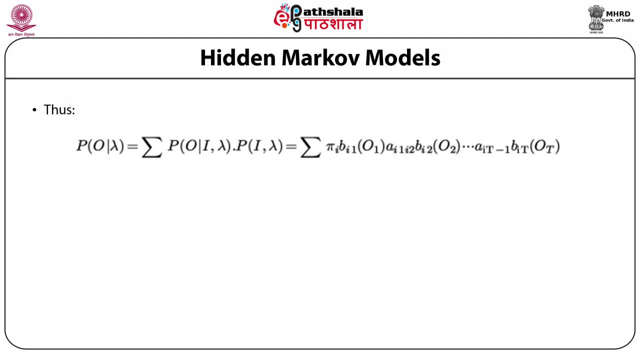 Now this is a fantastic equation, easy to derive. it turns out that this is extremely difficult to calculate. So if you have n states, n possible symbols in t different states, then to evaluate that equation you will need n to the power t calculations. Now that is really too huge. So in 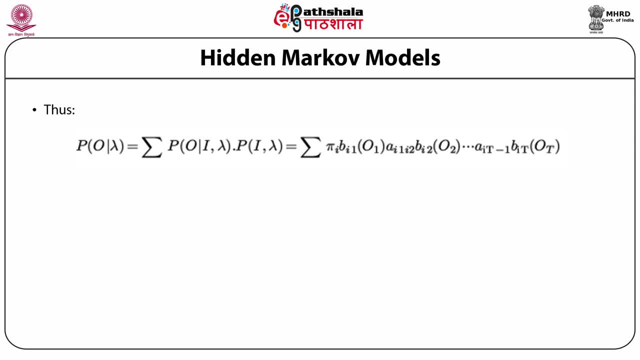 practice, this direct solution method is not used. What we have instead are two algorithms, basically the same algorithm, how you look upon it. One is the so called forward algorithm and the other one- it's dual- the backward algorithm, which simplifies this equation and gets you that probability. 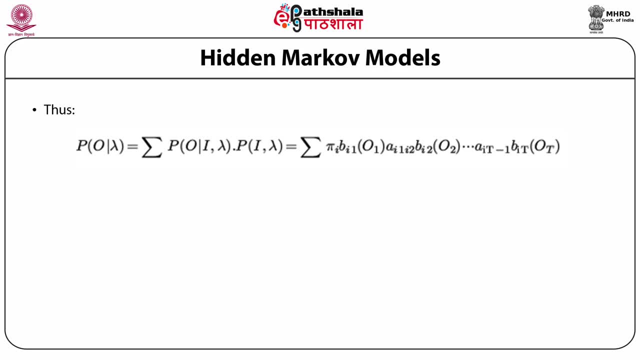 in a lesser number of steps, which make it more easier to calculate. So, in general, whenever you hear the evaluation problem, what is the probability that this sequence belongs to this Markov model? The answer would be: forward algorithm or it's counterpart, the backward algorithm. you can use any one, So that algorithm is what we are going. 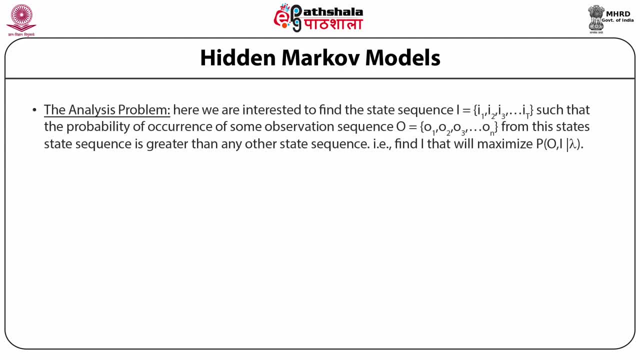 to use to obtain that probability? Now, if you look at the analysis problem here my question is slightly different. that I have a Markov model which has a certain state sequence within it, that I is equal to I1, I2, I3 and so on and so forth. Now, if I have an observed sequence, O is 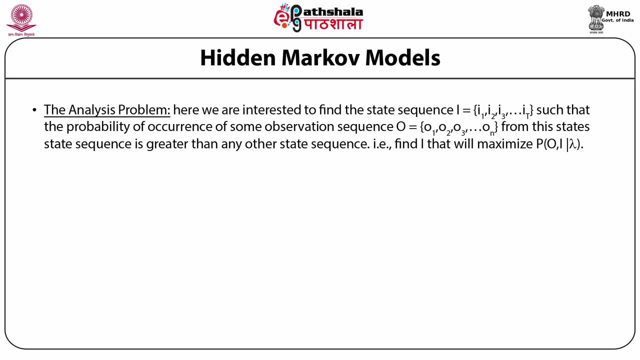 equal to O1, O2, O3 and so forth, so on and so forth. The question is: how well does that, the state sequence I predict the observed sequence O, Which means that I am asking the question: What is the joint probability of having the observed sequence O and the state sequence I, given by Markov model? 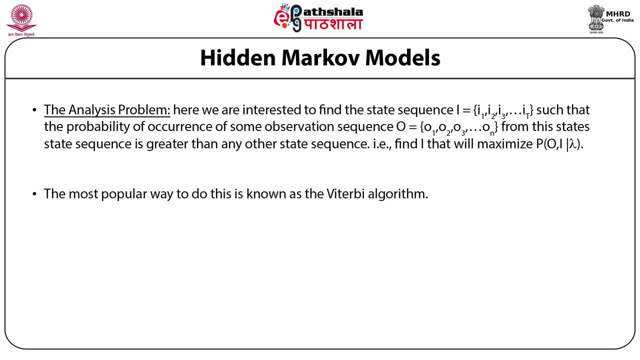 Again, the most popular way of doing this is called the Witterbe algorithm. I will not describe it much, the mathematics behind it, excepting to say that it is a kind of dynamic programming. and AND: Como es en rose apres yado twitter legando en Audiilanö. 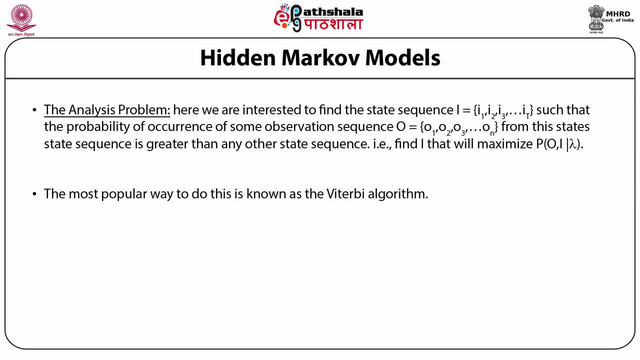 You are treating other the mathematics behind it, excepting to say that it is a kind of dynamic programming alright algorithm which you have seen when we are doing Needleman Wunsch and Smith Waterman algorithms during the alignment section. So it is something somewhat similar to that we 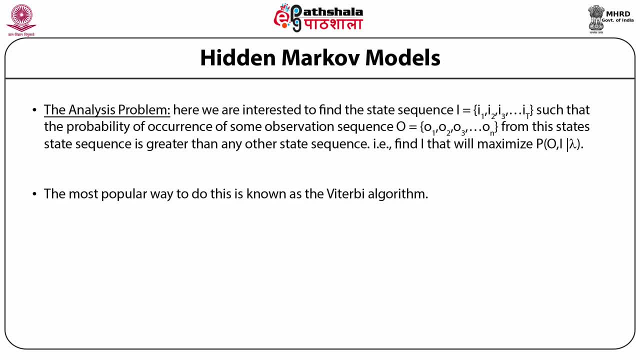 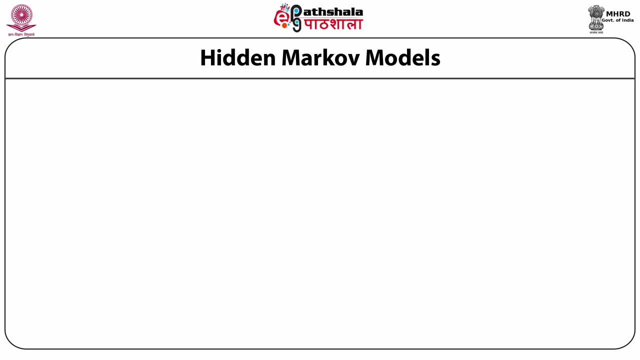 have this Witterbe algorithm which finds out this, the joint probability of my observed sequence and some state sequence I within my Markov model. and what I am interested is in finding the state sequence I. and then, of course, the last and most important thing is that how do I construct my Markov model? So this is the problem which trains the HMM. 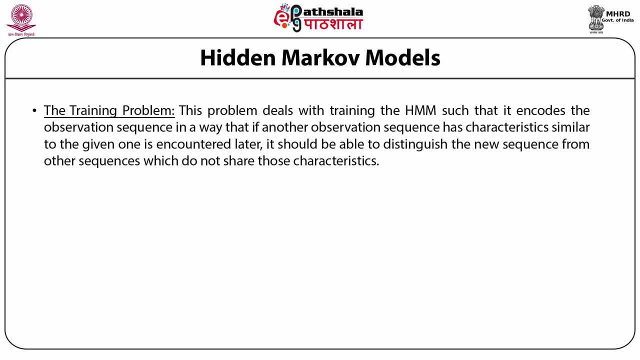 You give it a lot of data as part of a training set, and then you create the HMM from nothing. Now, the way to do it. we have an algorithm called a Baumwelsch algorithm, or sometimes also known as the expectation maximization algorithm, which is an iterative algorithm. 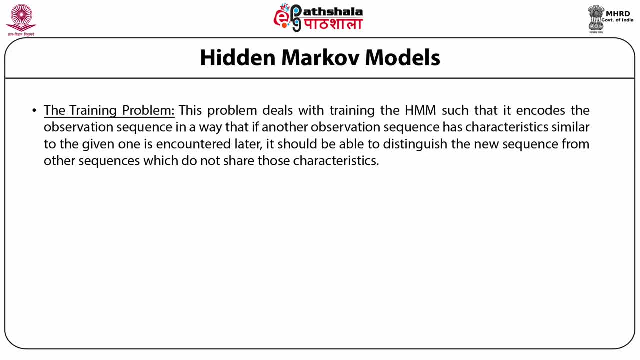 which starts one step at a time and repeats that step many times until convergence, and which is then used to create HMM and trained HMM. So again, summarizing the situation, what we have, that we have this Markov models, which essentially gives you a probabilistic view of a certain event, which 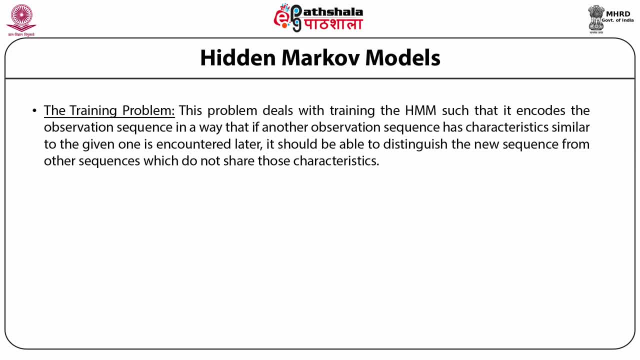 may be occurrence of a sequence or maybe so many other things. Now, given such a Markov model, we can ask a few questions. that our sequence or our event? what is the probability that it can be predicted by a particular Markov model, so called evaluation problem? Answer to that is the forward algorithm. 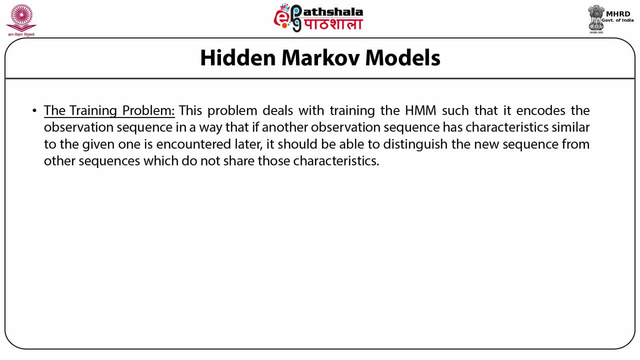 Second question: we can ask that, given this particular sequence fits this particular Markov model, is there within that Markov model a certain state, sequence i- which best predicts observed sequence? Basically, I am breaking apart my Markov model and finding out something from inside it, So we will call it the analysis problem. Answer to that, the solution to: 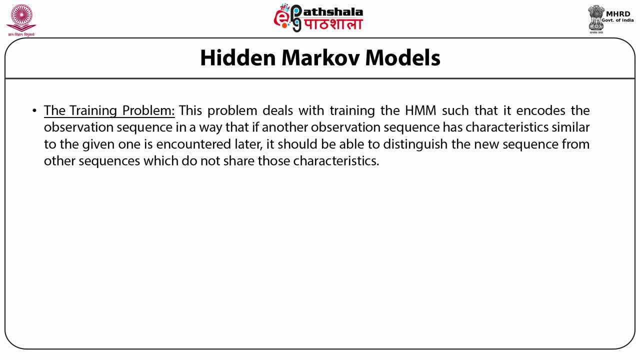 that is the Witterby algorithm. and finally, the last question is that, okay, how do I get my Markov model? So how do I train it, given certain training data, the method to train, that is the Baumwelch or the expectation maximization algorithm and that can be used to train a Markov model. So these are. 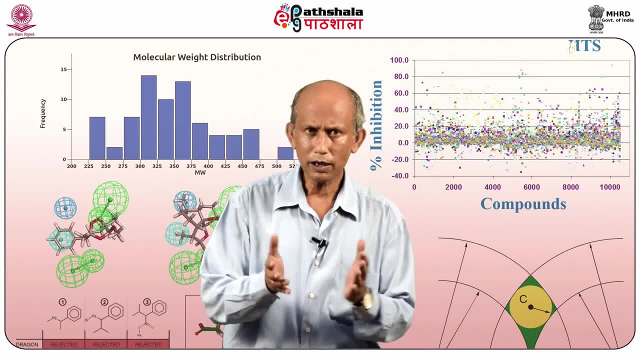 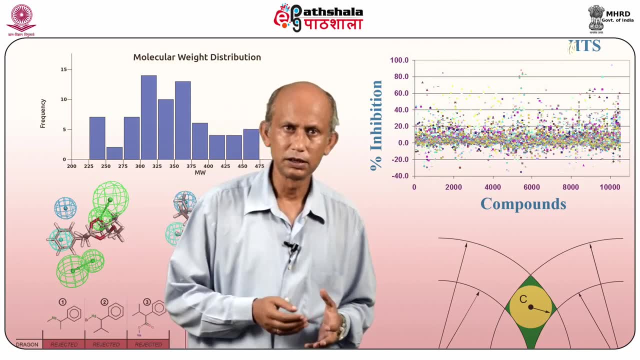 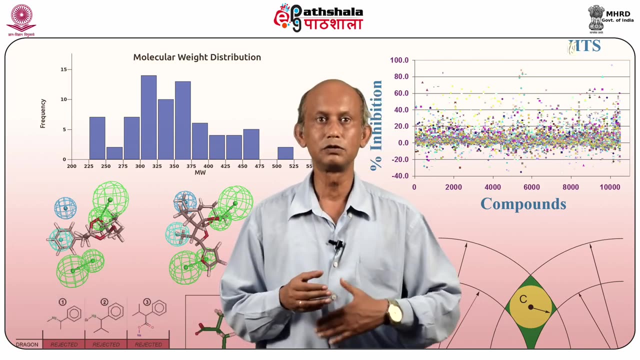 the three problems and there are three solutions. So, while the hidden Markov models which I have been describing thus far have come a long way, they are really very powerful methods. Now for biological sequence analysis. a little bit simplification can always be obtained, something which we call the profile HMMs. Now again, we know that biological sequences often come in families. 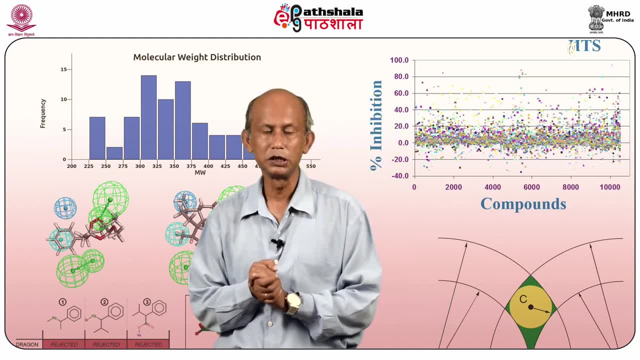 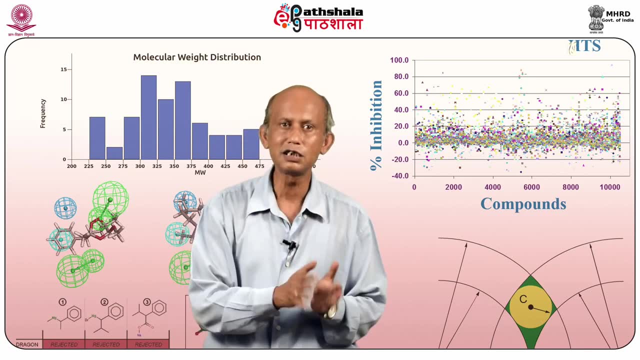 and the purpose of many a sequence analysis tool is to uncover the relationship between a particular sequence and its own family, or to discriminate between different families. That is what we have been talking about with our multiple alignments. We have been talking about the same thing about the 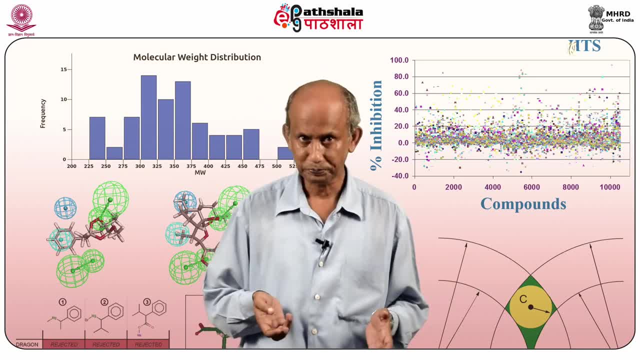 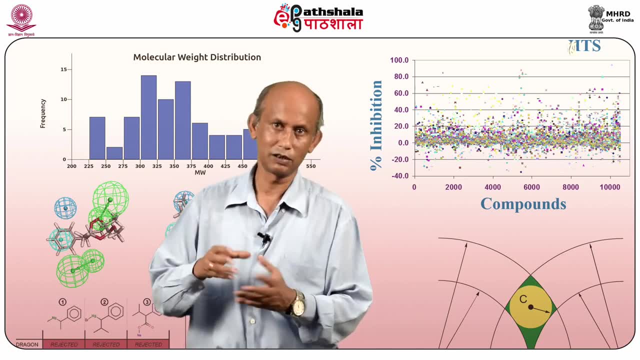 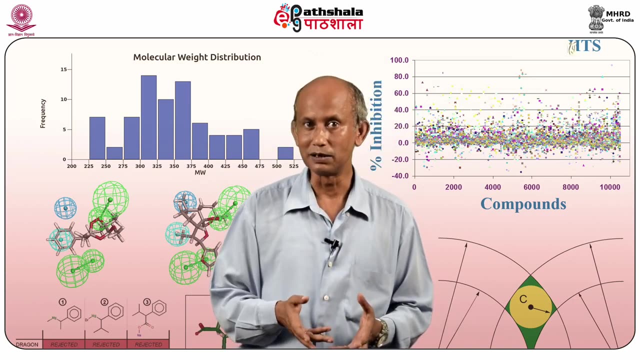 HMMs- we are talking with our profiles- or PSWM s or what not. So if one already has a set of sequences belonging to one particular family and one can do a database search with this family, we can uncover more members of their sequence family and to do this again, a kind of Markov models call. 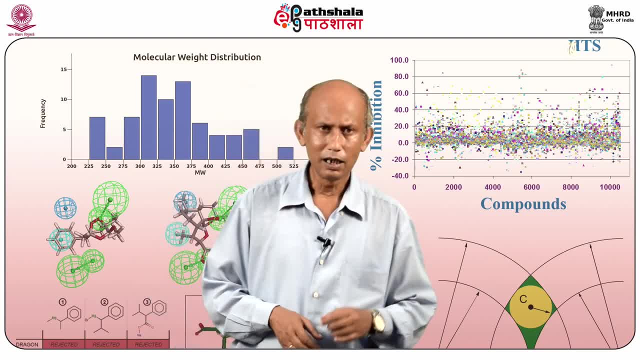 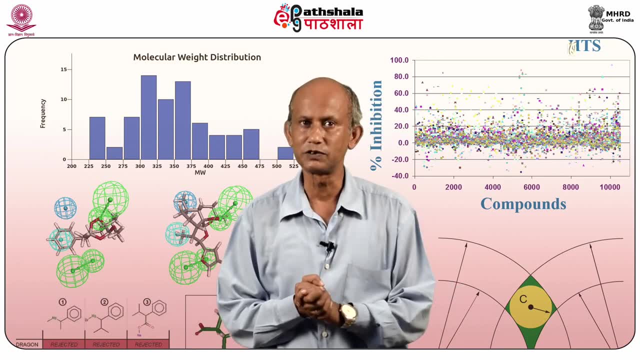 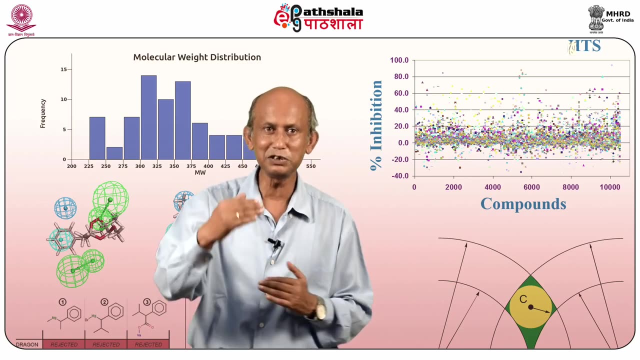 the profile HMMs can come in quite handy. So again, we have seen this before that a multiple alignment captures many characteristics of a sequence family, and if you can take the entire Markov multiple alignment and use it as a database search, it would be a pretty useful thing. 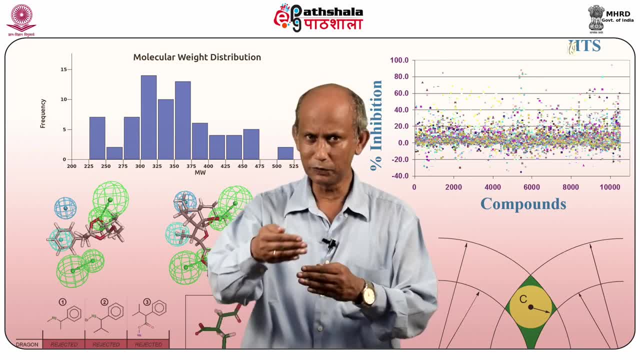 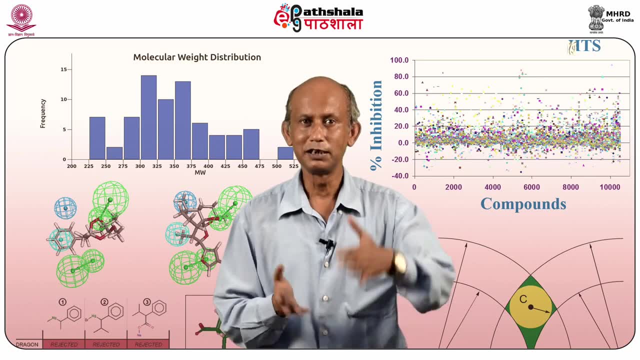 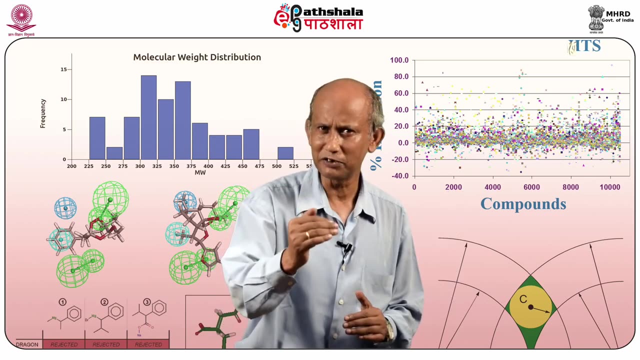 to unearth more members of that family. Just if we look back a little, that we see that our sequence motif, essentially what it does, it condenses a Markov multiple alignment into one motif. If we look at our weight matrices, what it does essentially takes a multiple alignment. 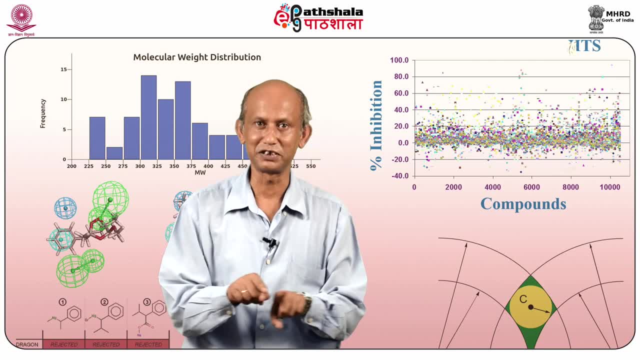 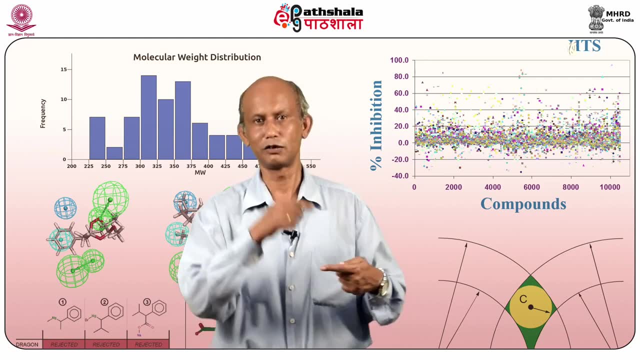 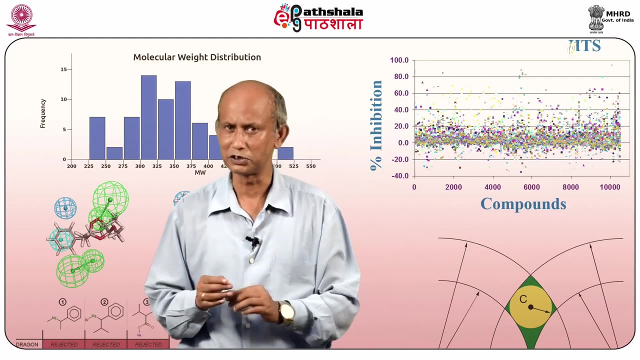 calculates the frequencies and tries to represent it. Now, in case of our motif, we had the problem that just amino acids are present there or not there. That's all we have. We do not have the frequencies. In case of the weight matrices, we do have the frequencies. so in that sense it's better. 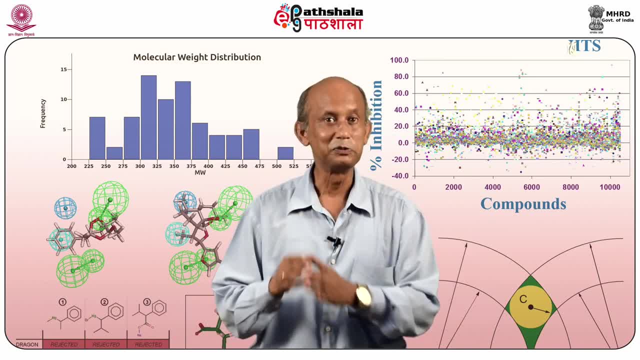 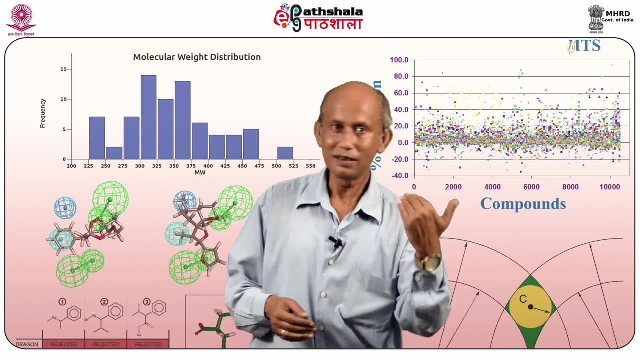 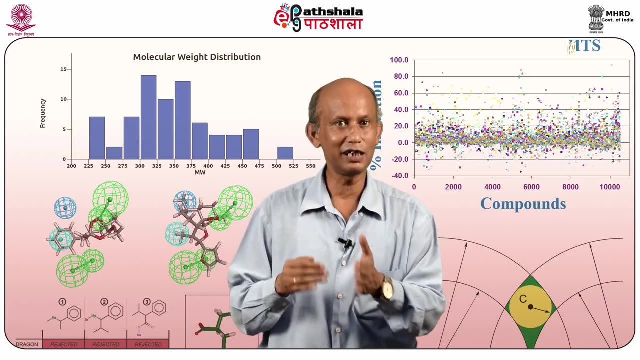 than the motifs. but it has a problem. We cannot handle gaps. Now we bring in the HMMs, which would be just like PSWM, but at the same time now we will try and model gaps. So again, these three things, the motif, the PSWM and the HMM, all of them take as their. 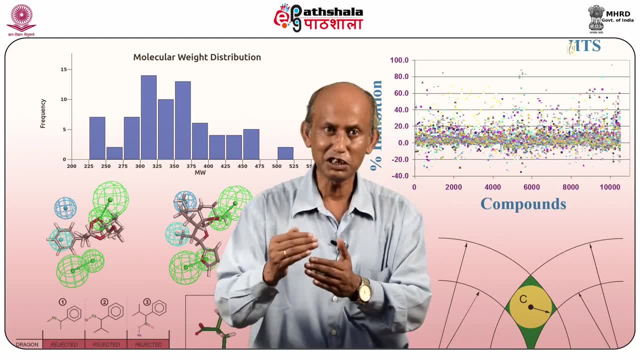 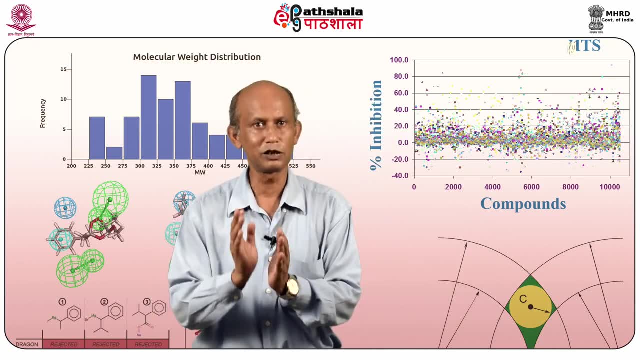 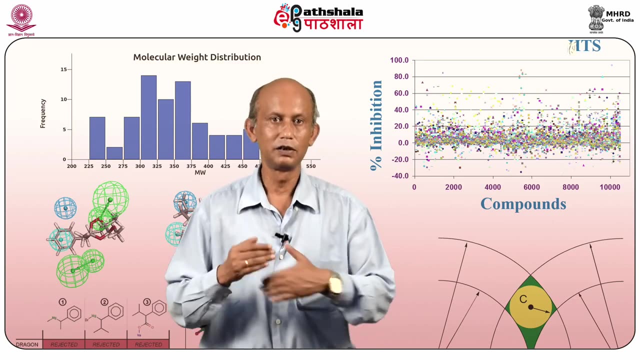 input, a multiple sequence alignment, but they treat it at different level of detail. At the lowest I have a sequence motif, very little detail. What more detail? is a PSWM? Okay, HMM, with a lot more detail. and how is it that it's handling both the amino acid frequencies? 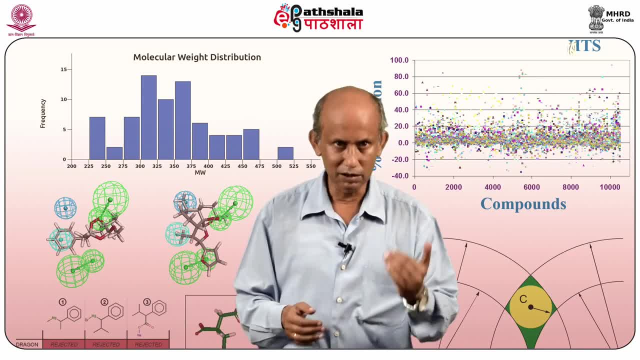 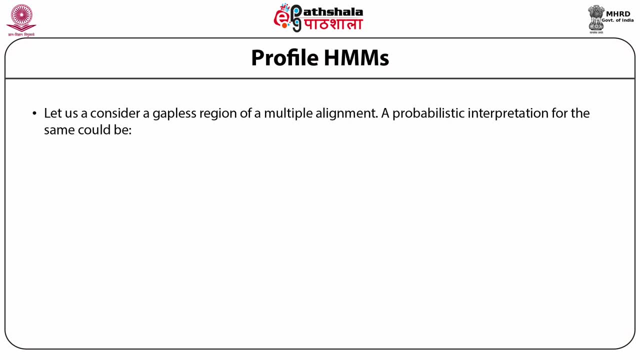 within the alignment, as also the gaps, etc. This is what I'll see next. So let's start with a gapless region of a multiple alignment and let us try to make it a probabilistic interpretation. So again, I can define the probabilities EI of A for observing amino acid a at a position. 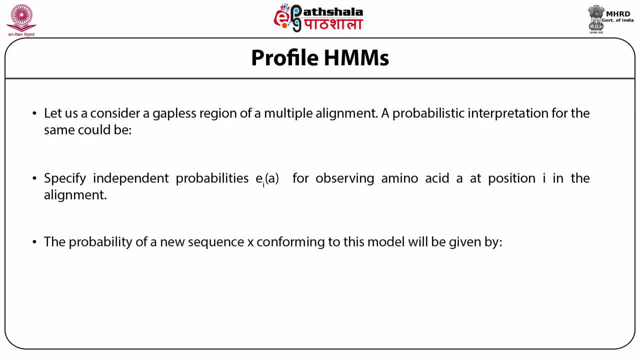 I in the alignment. So the sequence x, which conforms to this model, that is, px given n, will be the product of all of these eis for all of these positions that I have got. So that is the equation over there. Now, the ratio of this probability that x belongs to a particular family as opposed to x belong. 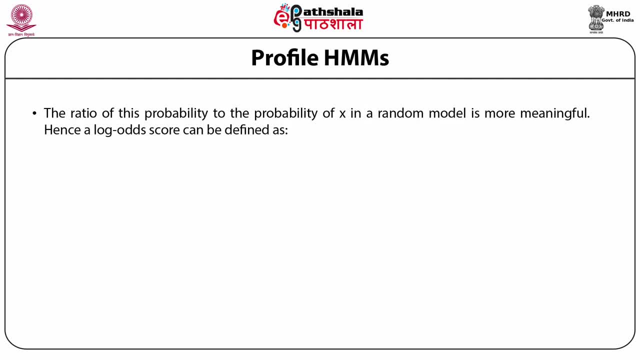 to a random model. again, I can use a log out score and I can define: s is equal to log of ei over q and instead of the product, since it is in the log scale now it will become a summation. So I have this particular formula Now. these values, the log of eia over qi is: 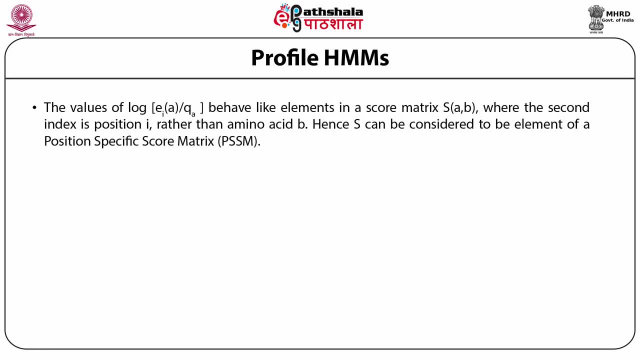 nothing but the pswm, right? So I can call it nothing but a score matrix sa of b, where the second index is the position rather than the amino acid. So these things will call it the position specific scoring matrix. Now a pssm can be written as the position specific scoring matrix, Now a pssm can be. 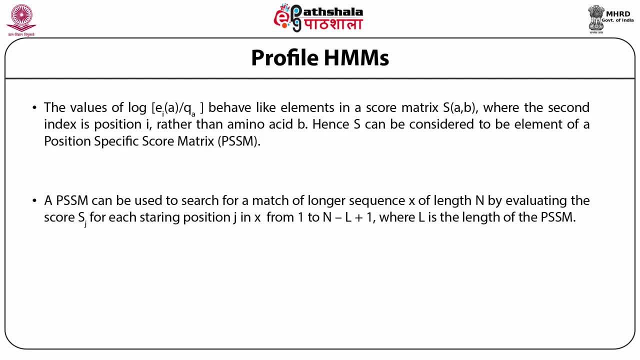 used to search for a longer sequence x in a database. Again, the function of this is exactly as a weight matrices operate. Everything is there because it is still not handling gap. So if you can now upgrade the pssm a little bit to handle gaps, then I go one better. 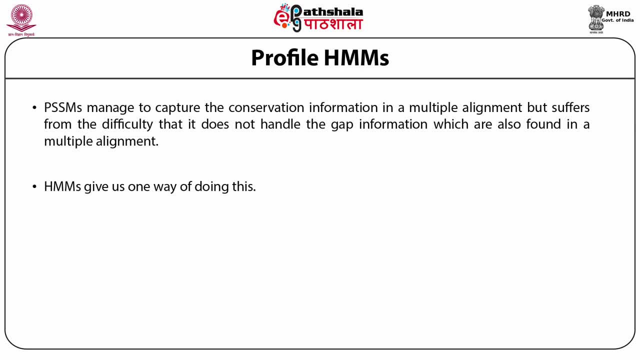 So one way of doing this, of course, is using hidden Markov models. How do I do it? So I can view my pssm as a very simple hmm, Which is just consisting of a sequence of states. So I have a begin state and then I 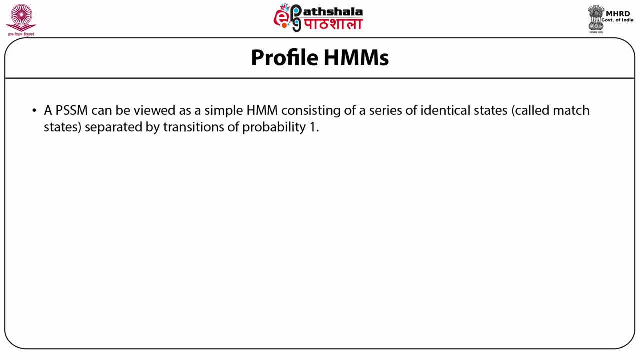 have. for each position in my pssm I have a particular state, a, b, m1, m2, m3, mj and going and ending in a particular end state. The emission probability of an amino acid at each of these states is simply the frequency of amino acids at that particular position of 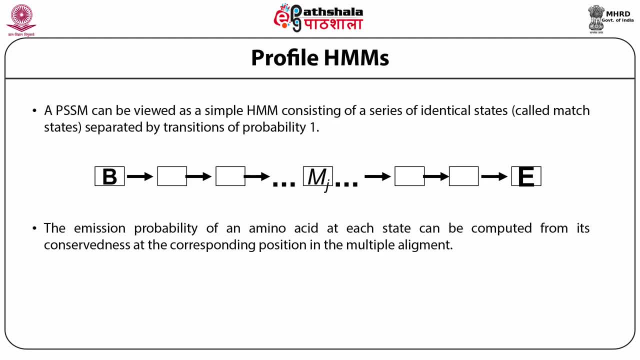 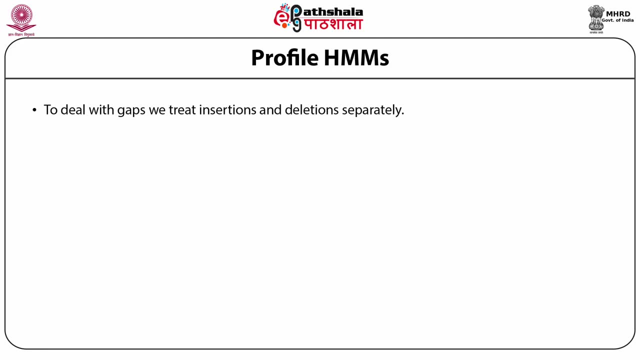 the pssm right. That is fine. So how do I know to handle gaps? I can think of them as handling insertions and deletions. I have to add additional states, So we model insertions and deletions as new states. For insertions I will between a state. 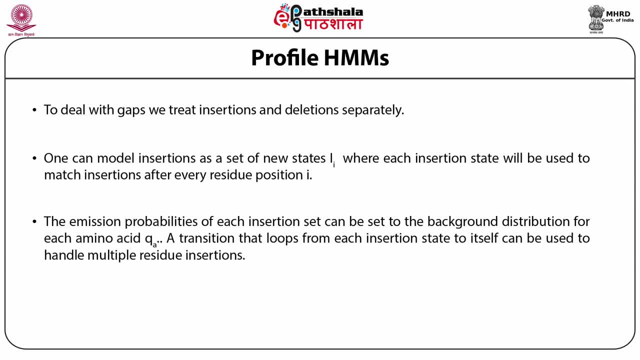 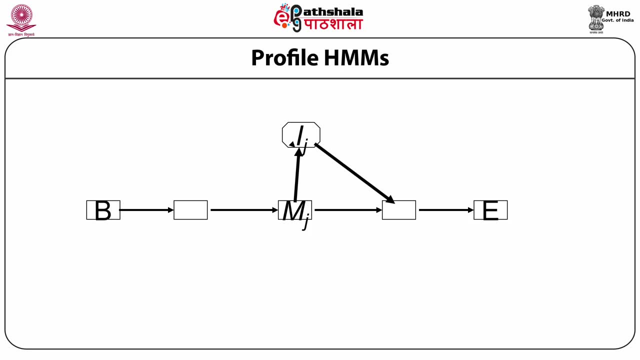 i and state j. I will now create a state k in between them with transition probability going from i to k, as well as i to j and k to j, Again from the state m j to m j plus 1. an insertion state now from m j. you can go either way. so in some of the sequences from m j you will. 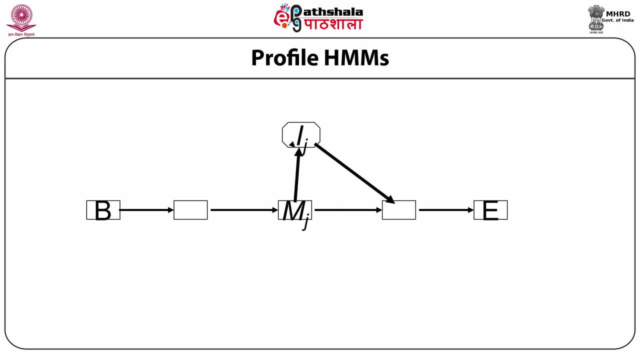 go straight away to m j plus 1, but in some of them from m j you will go to i j and then move from i j to m j plus 1. so where you are going via i j you are having an insertion where you are going. 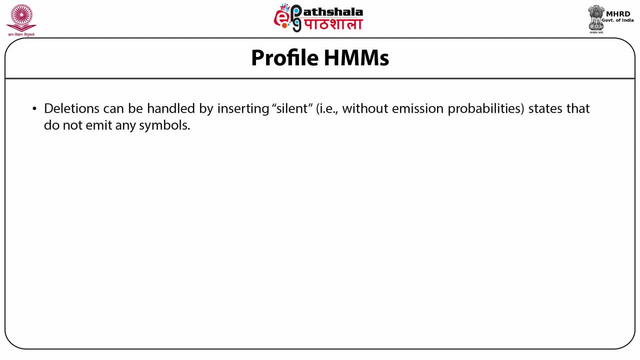 direct. you do not have it, so deletions are handled in this similar way. by now we will have some silent states which do not have emission probabilities, so let us call them d okay, and the cost of a deletion will be the sum of going from the match states, m states, to d states, and 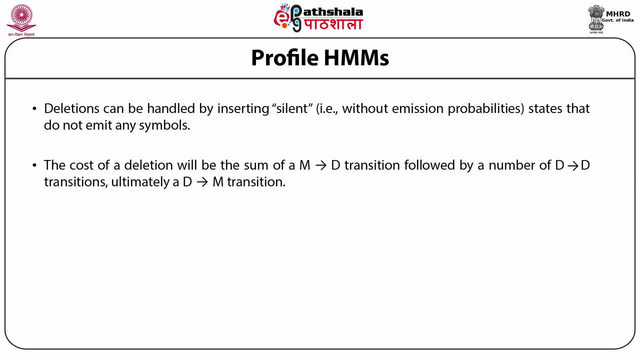 then there can be more than one d states, so you can go from one d state to the another and that transition probabilities can be again trained so as to handle different kinds of gap penalties. so this process can give us all kinds of gap penalties. you can use an affine gap penalty. 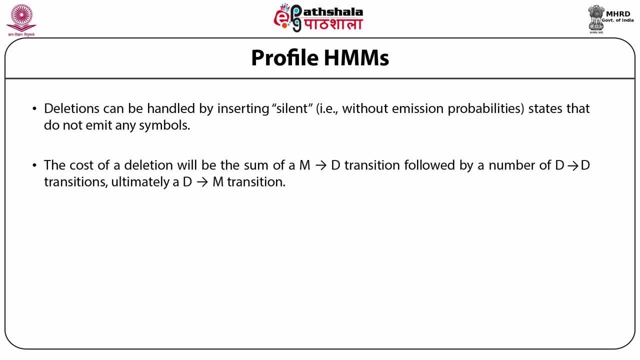 we'll try and train it in a different way, so this process can give us all kinds of gap penalties in a certain way. you want to use even a complex function of gap penalty. we can do that. so any arbitrary gap penalty model you have can be trained by adjusting the transition probabilities. 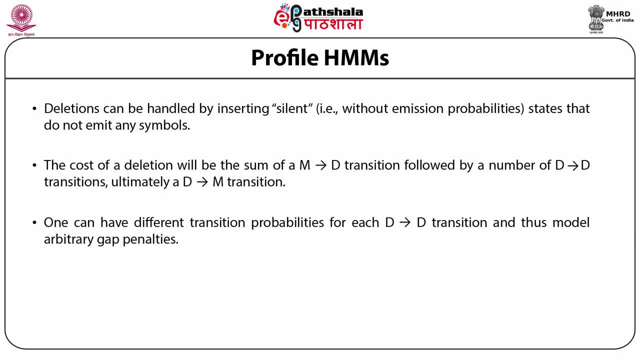 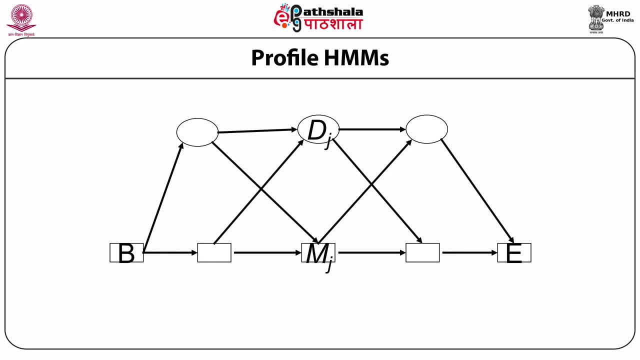 of the delete states to the delete states within your markov model. so here is an example of a basic match state with several delete states and the transition probabilities are given. now, as you go from one d to the another d, you can set the transition probabilities, thereby modeling. 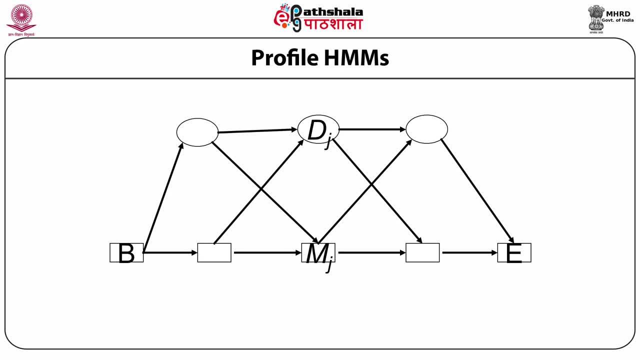 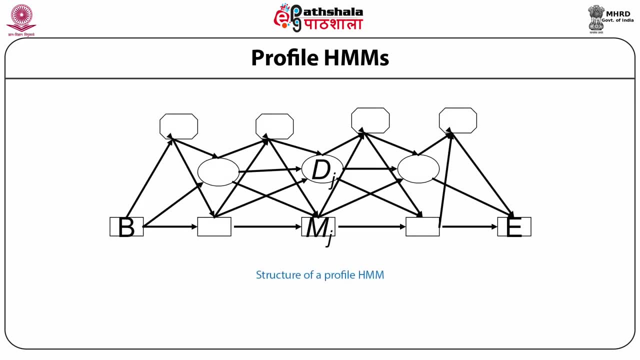 different gap penalties. so here is an example of a basic match state with several delete states. so this is the combination. so i have my basic match state model. on top of it i have both the insertion states and the delete states, so you can move any which way now. please note that once you. 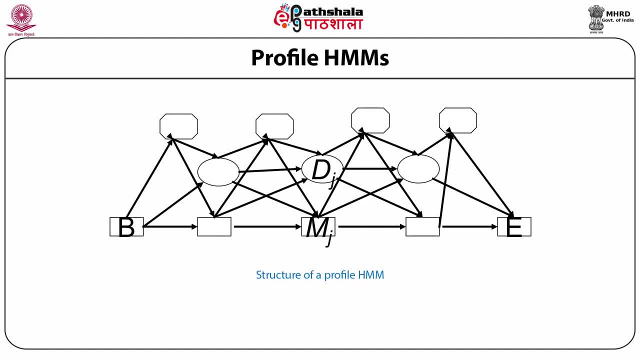 move into a delete state, you again come back to the match state, and so on, so forth. so in this way any arbitrary sequence which may have gaps, insertions or deletions can be now modeled within our PSsms. so this sort of hidden markov model is called a profile HMM, and this is a very 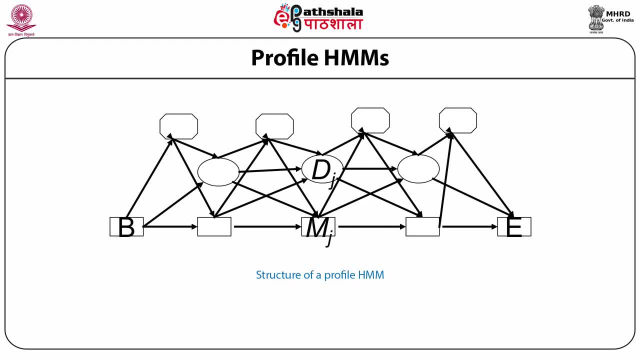 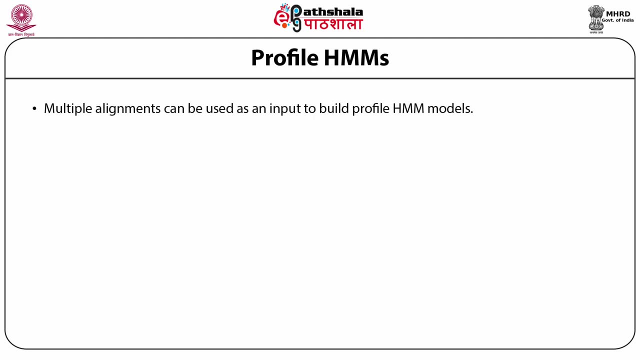 powerful tool and once you have trained a profile HMM on on a particular family of proteins, you can use that to search any other sequence, whether it belongs to that family or it doesn't. so again, for all such profiles HMMs, the input is a multiple alignment, the same way as it is used in motives, our 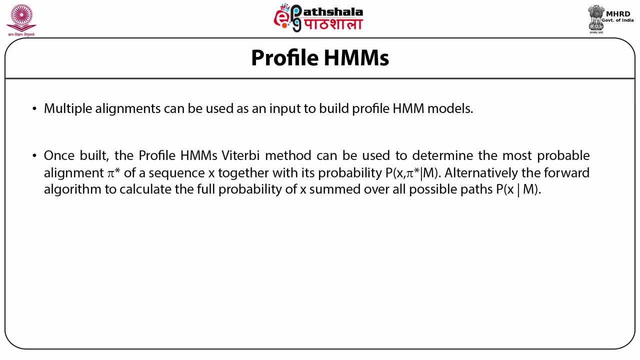 PsWm. okay, so once built, hmm helps with the conscious HMM effect. Robotics means when a of a particular value is changed between two properties. it incorporates a profile HMM and this Chicago a profile it HMM we can use to. they use the Viterbi algorithm to determine the. 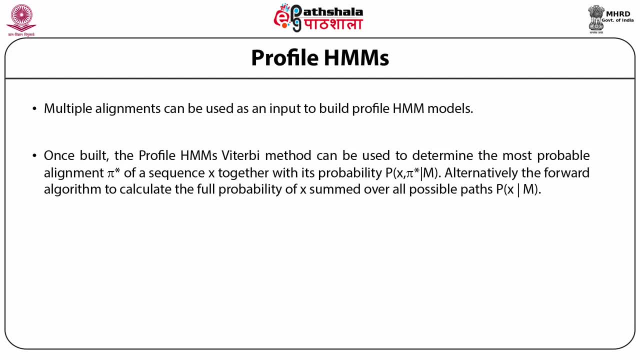 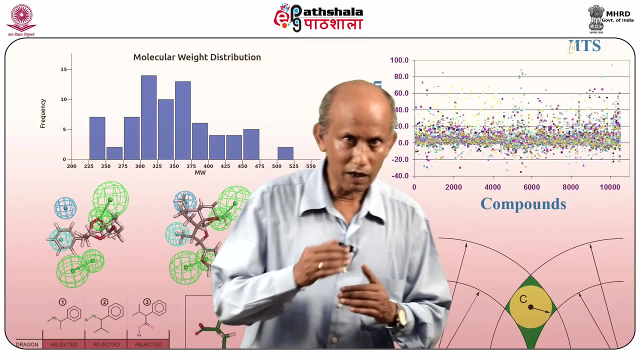 most probable state sequence within the that complex alignment, which would actually give me the alignment of a particular sequence to the rest of the family. alternatively, I can use the forward algorithm to calculate the probability that the sequence belongs to a particular family, summed over all the possible paths in the hidden Markov model. so, in summary, out here we have. 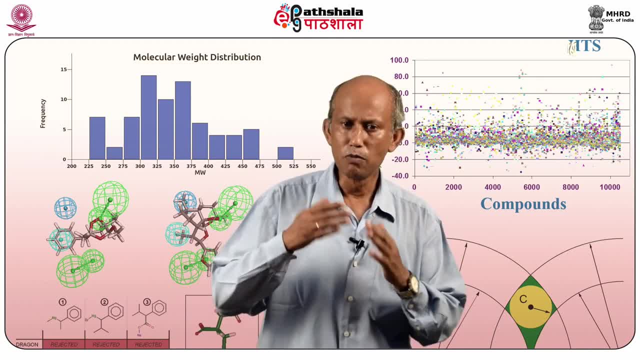 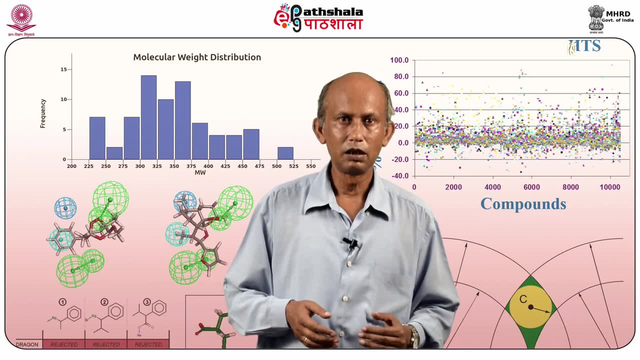 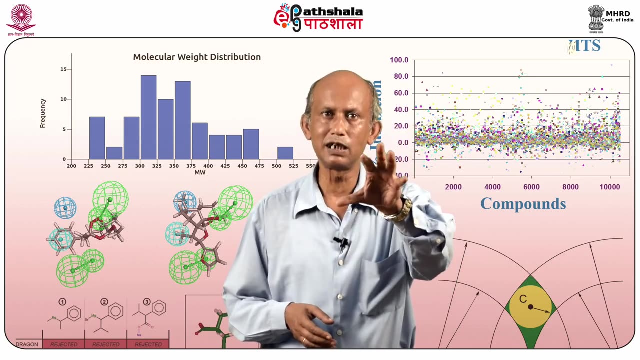 discussed in pattern recognition several methods. most of these methods, be it sequence motif, be it position, specific weight matrix, be it even, in certain sense, psi blast, what we have done, we have either used a multiple alignment as an input or, in case of psi blast, we created that multiple alignment on the